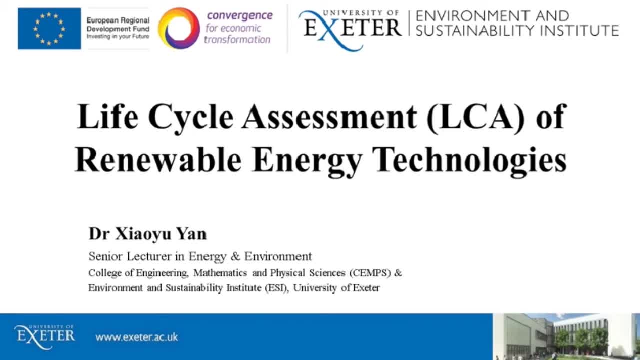 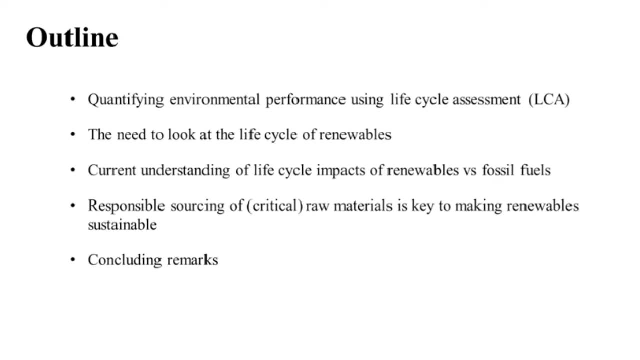 the effects of energy technologies and systems on the environment, and I'm really glad to have this opportunity to talk about an important topic, which is life cycle assessment of renewables. So here's what I hope to go through in the next 20 minutes or so I will. 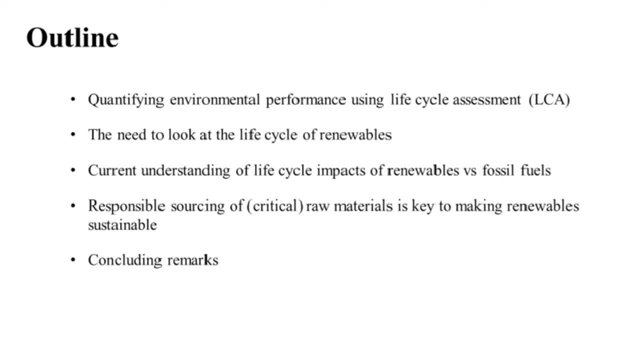 start with a brief introduction to the life cycle assessment method, or LCA, which is a key tool to quantify environmental performance of any products or technologies. We then look at why there's a need to use LCA to evaluate the renewable energy technologies. I will present the state of 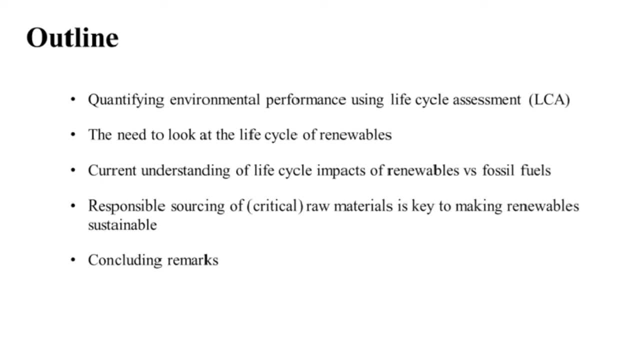 the art understanding of the environmental impacts of renewables from a life cycle point of view in comparison with fossil fuels. I will also talk a little bit about responsible sourcing of raw materials, particularly critical metals such as rare earths, because I think this is really key to. 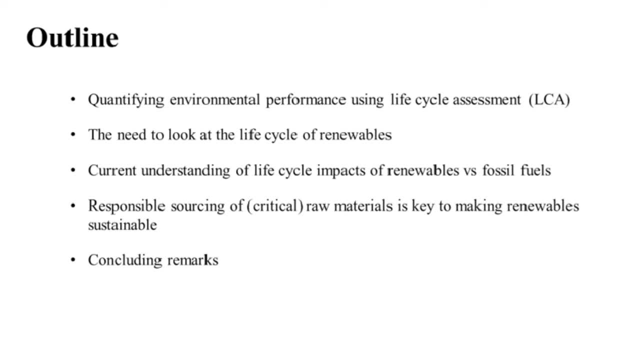 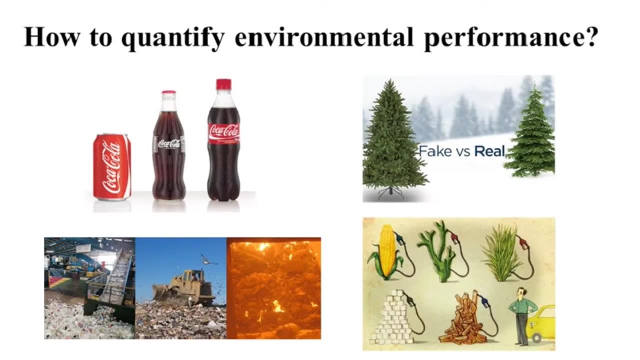 making renewables sustainable, or certainly more sustainable. And finally, I will summarize some take-home messages. We all know that we need to tackle the enormous environmental challenges facing humanities today, but in order to do so, we need a way to quantify and compare the sustainability of different actions we take every day as individuals. 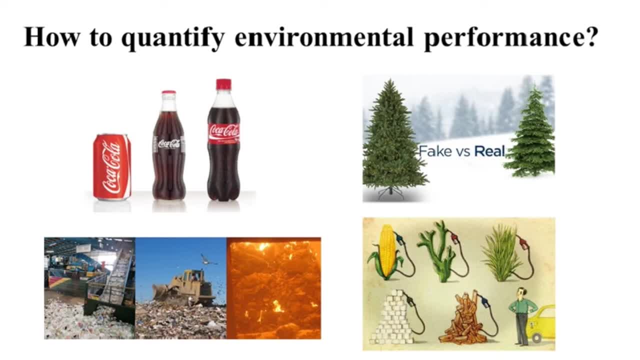 organizations and society as a whole. For example, companies might need to know which types of material is best for their products, or we as individual consumers might want to know the environmental impacts of things that we buy. At the society level, we need to know the best ways to deal. 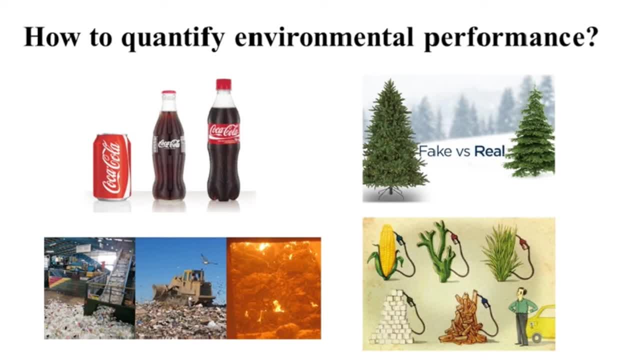 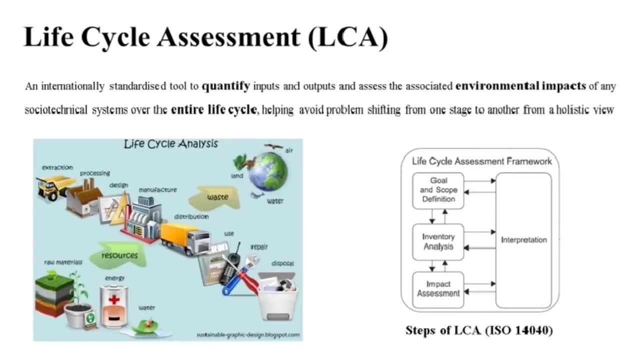 with waste. We need to know the environmental impacts of things that we buy. At the society level, we need to know the best ways to deal with waste and generate energy. So we really need a consistent and reliable method to do this, And this is where LC8 comes in. It's a standardized tool to quantify the inputs. 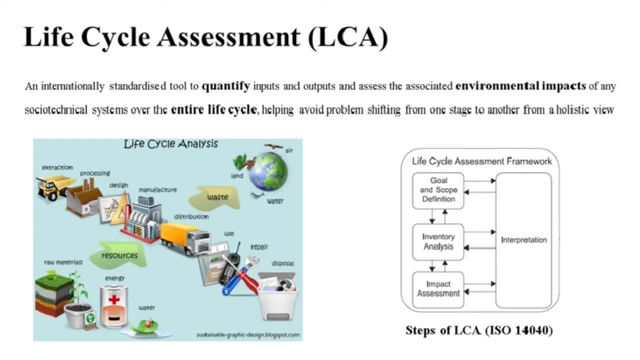 such as resources and outputs, such as waste and emissions of any product systems over their entire lifecycle, from the extraction of raw materials to the manufacturing, through to the end of life, and also assess the environmental impacts associated with these inputs and outputs, And this gives us a holistic view of the overall impacts of any defined system and therefore, 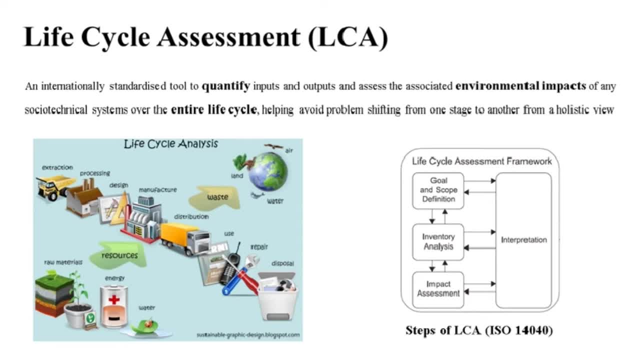 can help avoid problem shifting from one lifecycle stage to another or one place to another. And in the ISO standards for LCA there are four main steps. There's goal and scope, definition, inventory analysis, impact assessment and interpretation, which sort of runs in parallel with the other three steps. 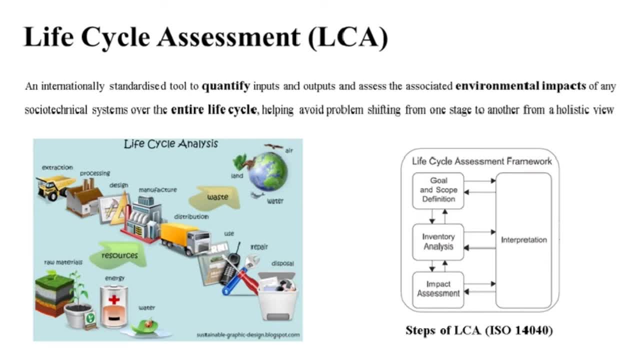 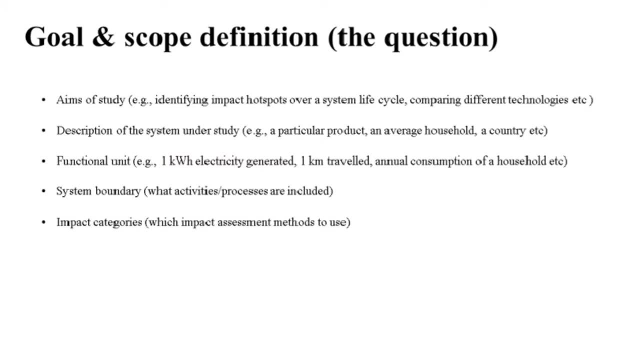 Now I will briefly go through how you go about doing these so that you understand what I'm talking about when I say lifecycle impacts of renewables. So the first thing of an LCA study is to define its goal and scope. You need to clearly state the A. 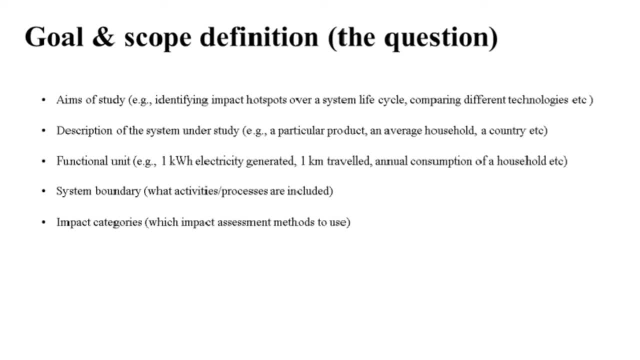 You need to define the aim of the study, which usually relates to a central question you want to answer, for example, whether a product is better than another, And describe the system you want to assess, especially if it's a new technology or new. 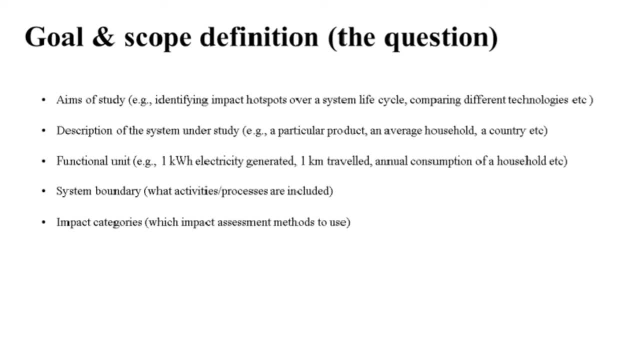 product. You then need to define the so-called functional unit, which is a quantitative measure of the main function of the product system And that provides a reference to which all the inputs and outputs are. And then you need to define the system boundary, which defines what technological and economic 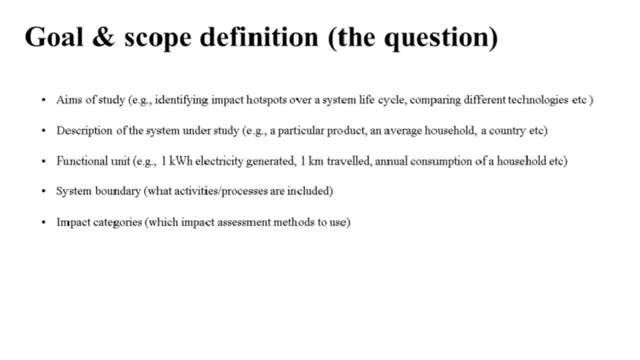 processes need to be included in your LCA And state which impact categories are of concern, because there are quite a lot of impacts that we can look at And also these will be included in your LCA. And also these will be included in your LCA. 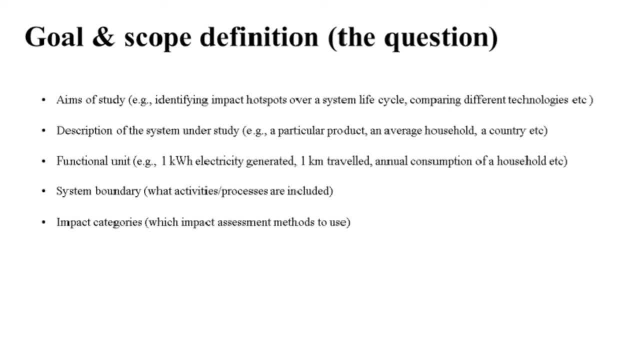 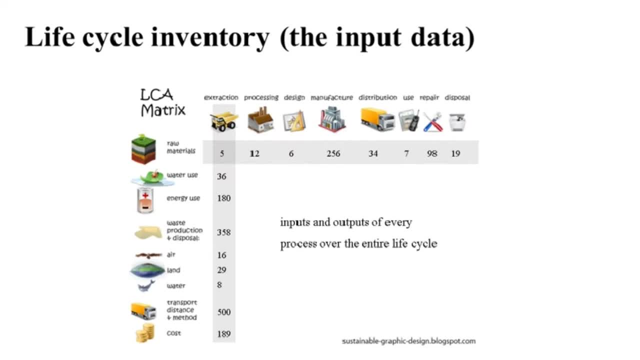 The second step is life cycle inventory analysis, or LCI. The aim of this stage is to quantify and compile all the physical inputs, such as different resources, required to a given product system, and the outputs, such as different products, emissions and waste generated. 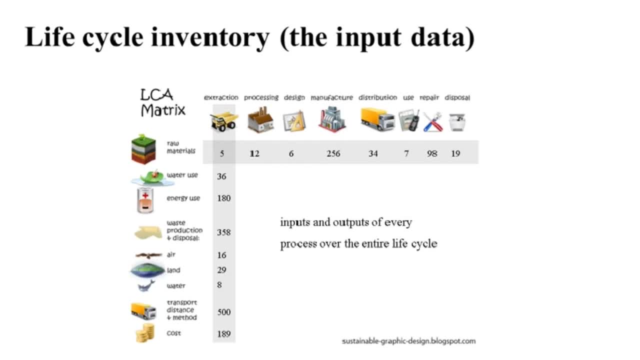 from the same product system. Now, this is usually the most labor-intensive and time-consuming stage, as there's a lot of number crunching needed. So essentially, you're building a very big matrix of inputs and outputs, as shown on this slide, And the third step is called 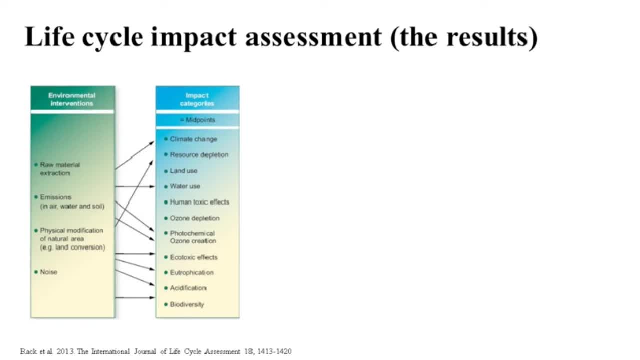 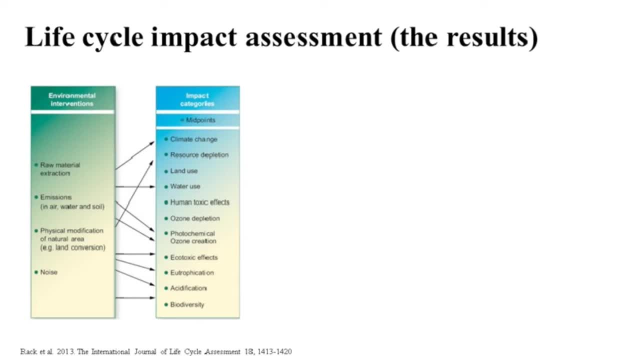 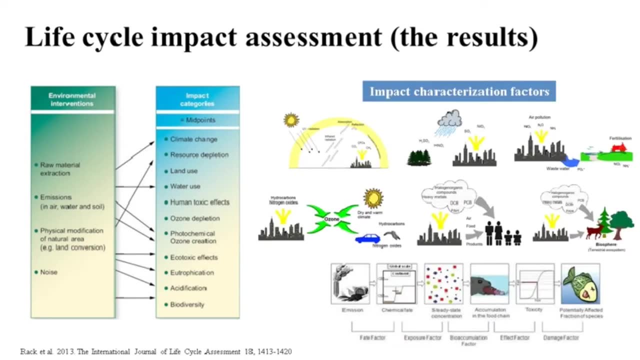 So this is a very important step. So this is a very important step of resource use and emissions into different environmental impacts including, for example, climate change, land use, water pollution, et cetera. And these characterization factors are usually derived from modeling the environmental mechanisms. 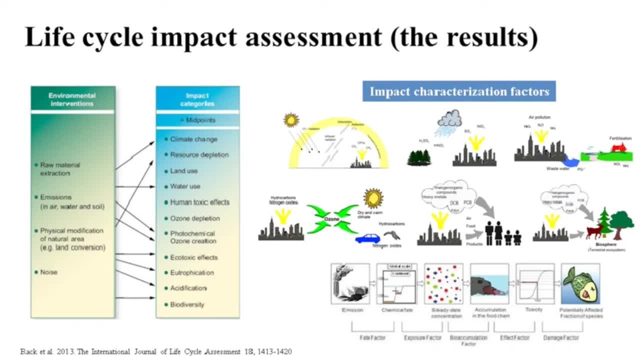 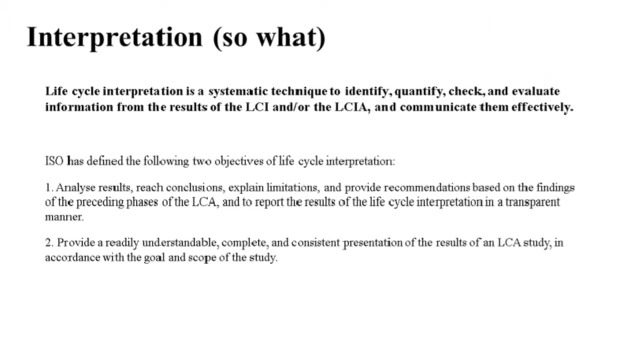 of a particular impact pathway based on our understanding of the complex system of physical, chemical and biological processes involved, And there are many different LCIA methods to choose from, so which one or ones needs to be used in a particular study depends on the impact categories of concern. And the last step of LCA is 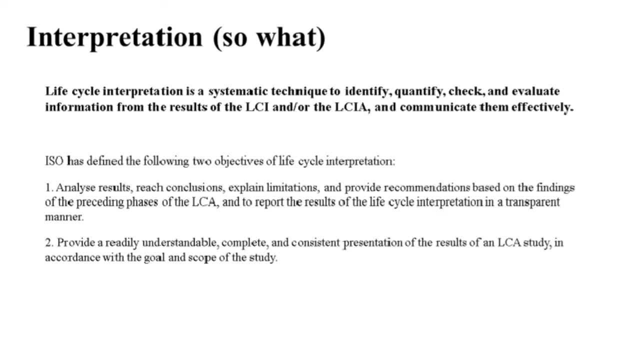 interpretation, and this is a systematic technique to identify, quantify, check and evaluate information from the results of the inventory analysis and impact assessment, and also communicate them effectively. So, basically, we calculated all these numbers. so what? What do they mean? Completing these four steps means: 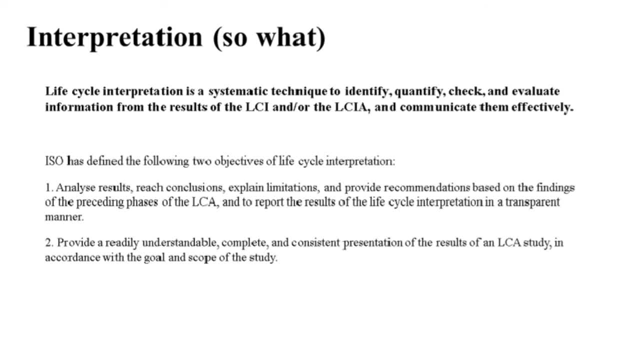 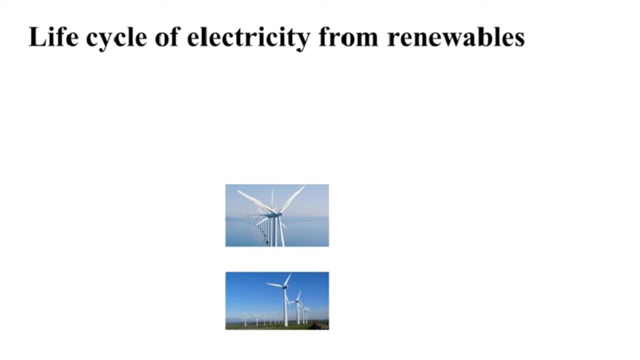 that you will have done an ISO compliant LCA study. Now you might wonder: why do we need to do an LCA? to assess renewable energy technologies such as wind turbines? Surely they have zero or minimal impacts? Well, it is true that during operation they are pretty clean. they don't emit. 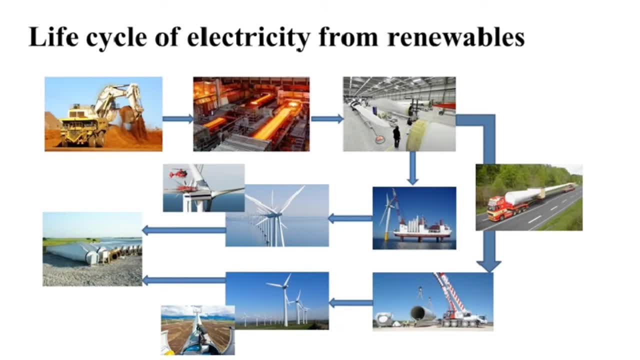 anything but over their entire life cycle. from mining the minerals and oils through to the raw material production, such as steel, glass, reinforced carbon fiber components, manufacturing, transportation, installation maintenance and repair and finally, decommissioning and disposal, every step of their life cycle will involve use of some sort of resources. 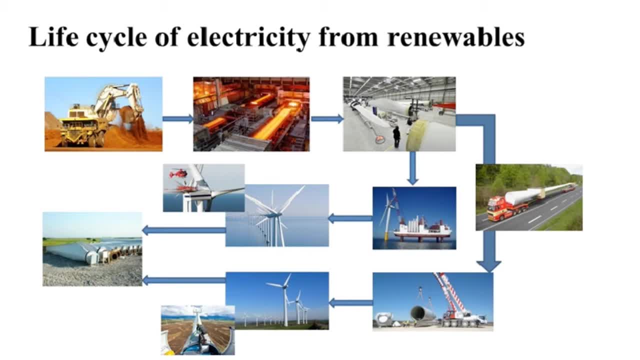 such as energy and water, and generate some waste and emissions such as CO2.. So they're not really zero emission or zero impact. It's just that most of their impacts do not happen at the operational stage and this is why we need a good understanding of their impacts in comparison with other energy. 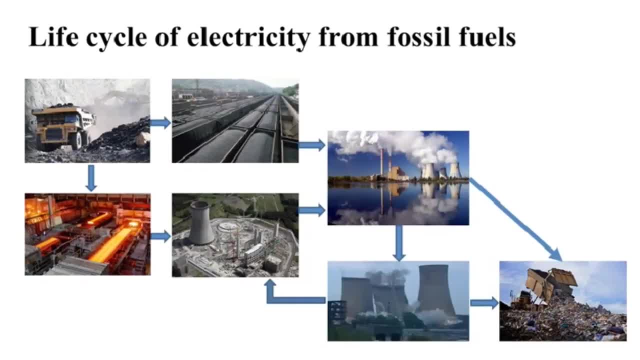 technologies such as fossil fuels. So if we look at the life cycle of electricity generated from fossil fuels such as coal, now this is relatively straightforward. You need to mine again the raw materials for your coal power plant and then you build the plant. You also need to mine and 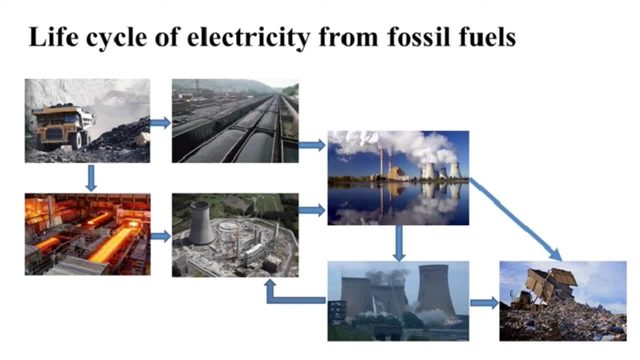 transport the coal to the power plant, and then it's the operation of the power plant, ie burning the coal to generate electricity, And of course, finally, the decommissioning of the power plants and then the demolition waste being either recycled or disposed of. So we need to use LCA to evaluate. 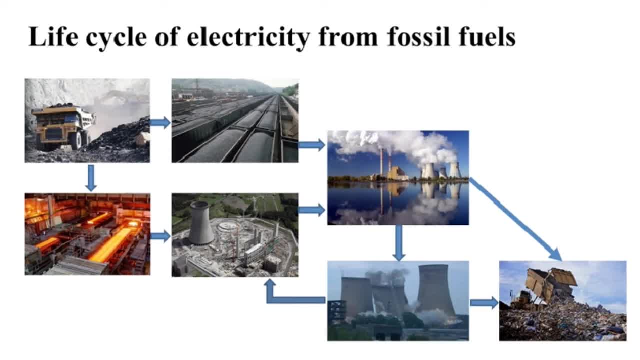 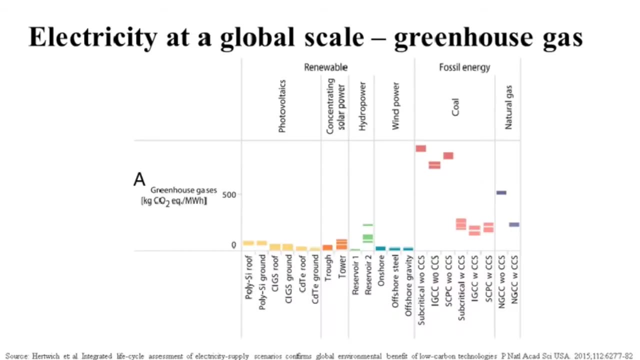 all the energy technologies to fully understand their impact, so that we can choose the ones with the best environmental performance in order to move towards a sustainable energy system in the long run. So now let's look at the next slide. Some results from some of the best LCA studies, comparing electricity generated from fossil fuels and 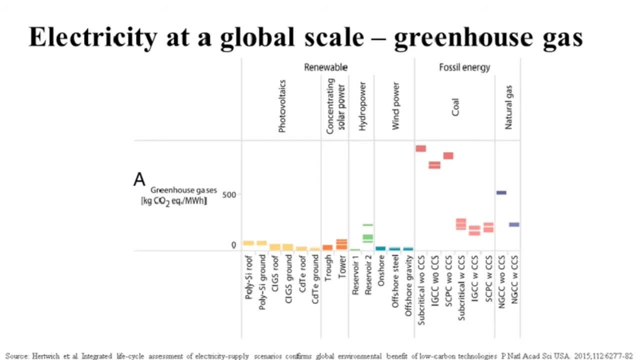 renewables. Now, in the interest of time, we will focus on just a few key impacts. only This global scale study, shown on this graph, found that the life cycle greenhouse gas emissions, also widely known as carbon footprint, of electricity generated from fossil fuels are much higher than that from renewables, as you can see there. So, for example, 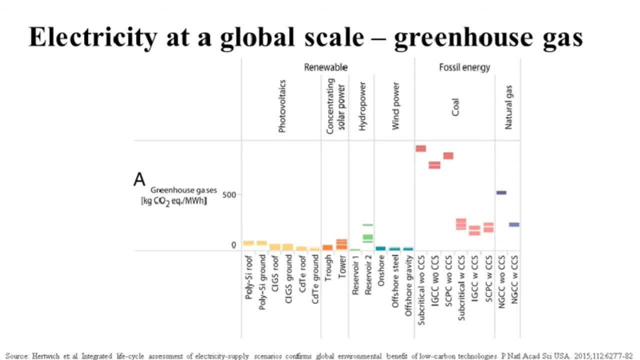 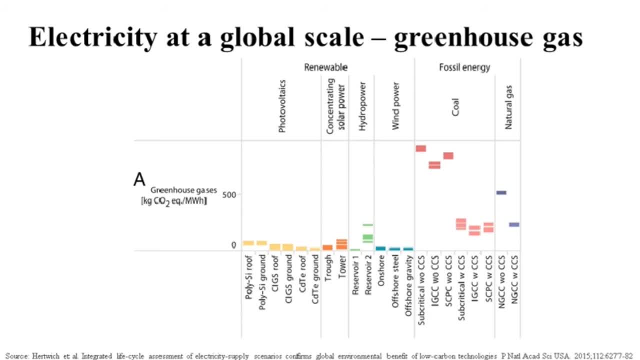 If you use carbon capture and storage, this can potentially be reduced to about 500 megawatts per megawatt hour. In comparison, pretty much all renewable energy technologies on the left-hand side considered in this study, including solar photovoltaics, concentrating solar power, hydropower and wind. 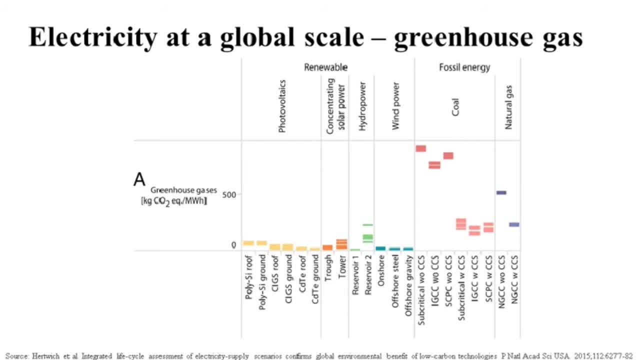 power are below 100 kilograms of CO2 equivalent per megawatt hour And, of course, as you can see, the only exception is hydropower, and this is mainly because the creation of reservoirs, particularly big reservoirs, can generate. 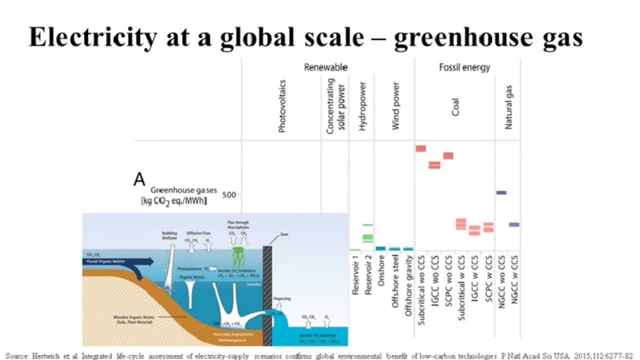 greenhouse gas emissions. So when a large area needs to be flooded to create a big reservoir, what happens is that the vegetation above ground and the soil, organic matter below ground will gradually decompose and release significant amounts of CO2 and methane, which is, of course. 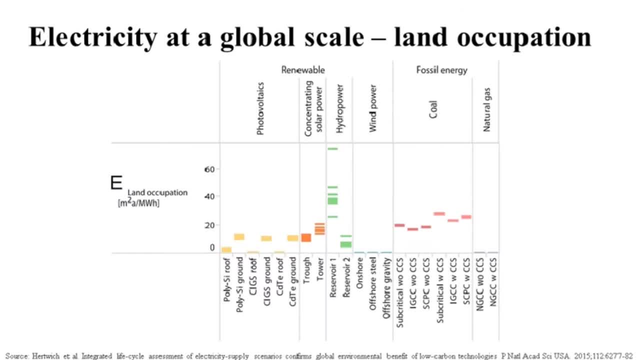 a powerful greenhouse gas. If we look at land occupation, which is a key driver for ecological impacts and biodiversity impacts, the same study found a very mixed picture. So, first of all, there's a big difference between coal and natural gas, mainly because of the nature of these fossil fuels and the methods used to mine or extract them. 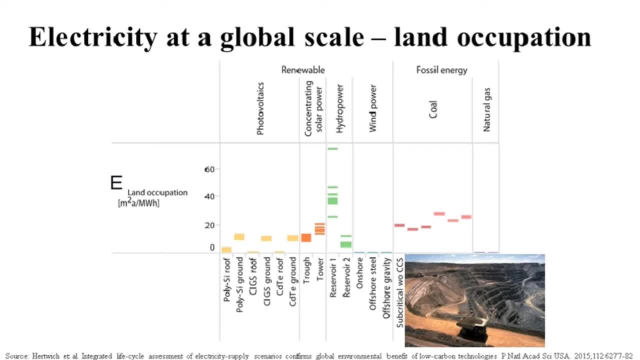 For example, if open pit mining is used, then the production of coal can occupy more CO2 than the production of rainwater, which can destroy the natural gas supply. Also, if you look at land occupation, which is a key driver for ecological impacts and biodiversity impacts, 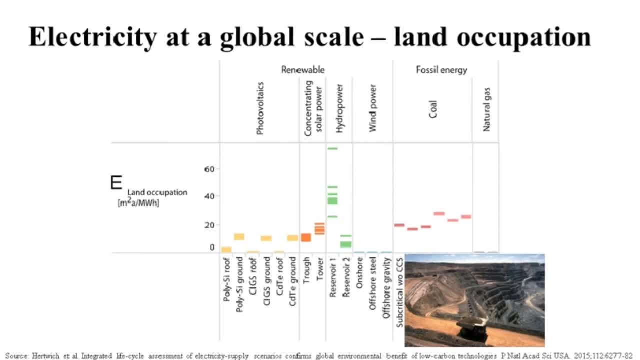 occupy a very large land surface indeed. The renewables vary significantly, from minimal land use by wind power to significant land use of hydropower, And sometimes hydropower can even have higher land occupation than coal, as shown on the figure. And again, this is because 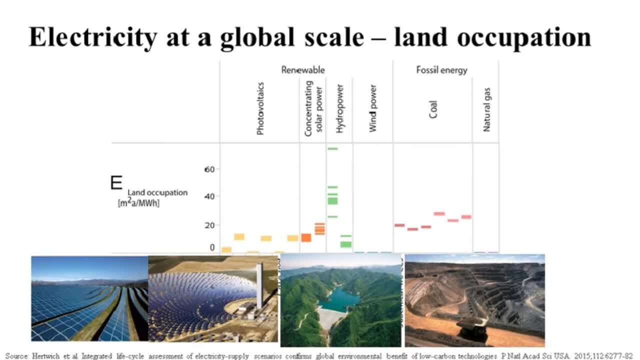 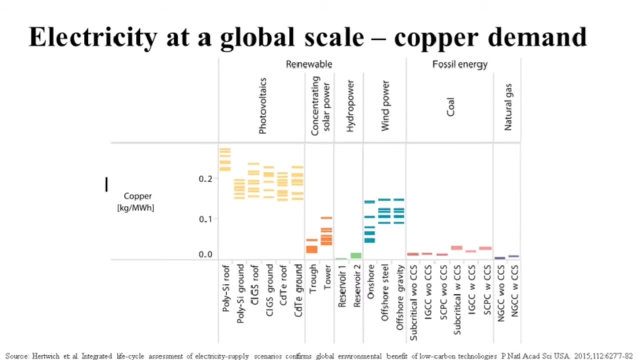 of big reservoirs, But for solar power, land occupation can also be very high if there are ground-mounted systems, such as ones shown on the photo on the left. Another impact is demand for metals that are heavily used in energy systems, such as copper. You can see that on a 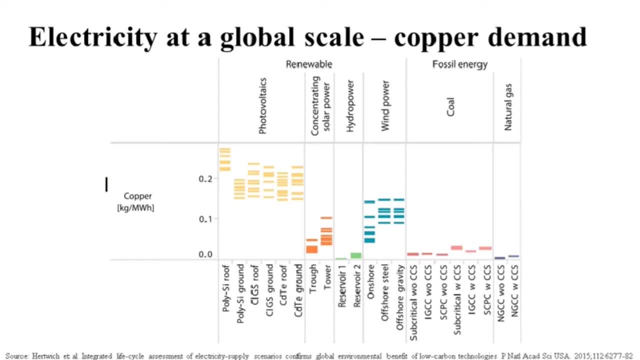 per-energy output basis, PV and, in fact, most renewables except hydro, have much higher demand for copper than fossil fuels, And this is mainly because more inverters and transformers are needed for these technologies, While demand for metals is not an environmental impact per se, but the mining and processing of 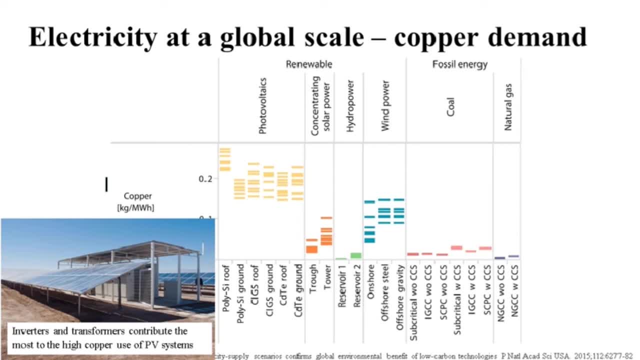 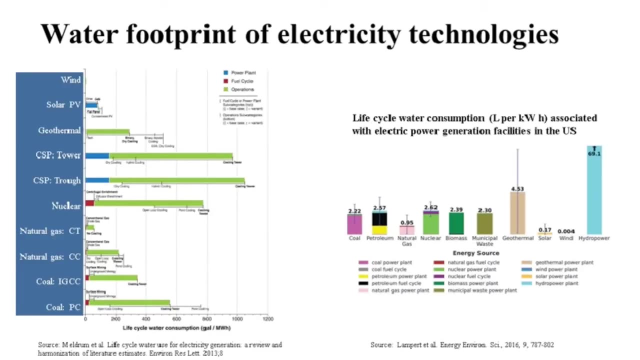 these metals are usually very energy and therefore carbon intensive, And they can also cause pollution of water and land. So we really need to have a good handle on this, And I will come back to this point later. Finally, water consumption is another key impact we need to understand. 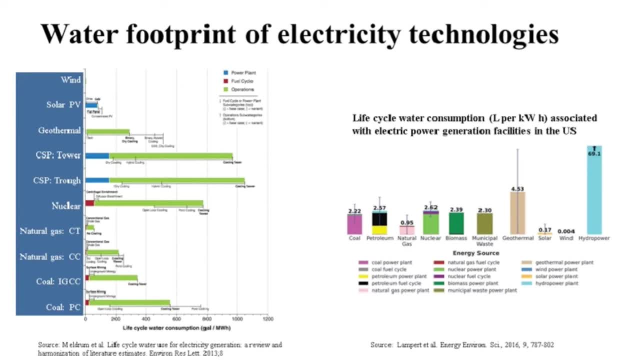 because water is an essential resources for humanity that is getting increasingly stressed because of climate change and pollution. So energy is actually a very thirsty energy industry And on the left you can see that any kind of thermal electricity generation technologies, including renewables such as concentrating solar power and geothermal, 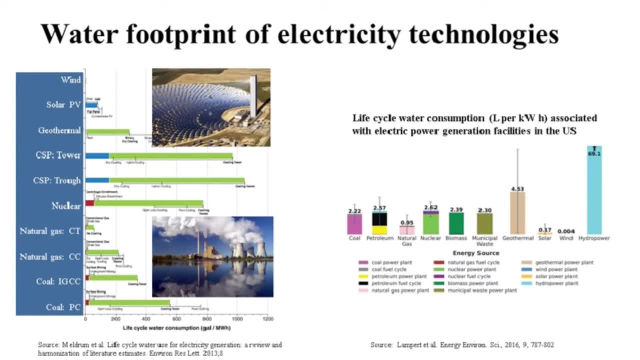 as well as fossil fuels and nuclear, can have a very high water footprint, primarily during the operational stage, because water is used as a medium to transport heat, as shown in the picture, And then, of course, we need to have a very high water footprint. 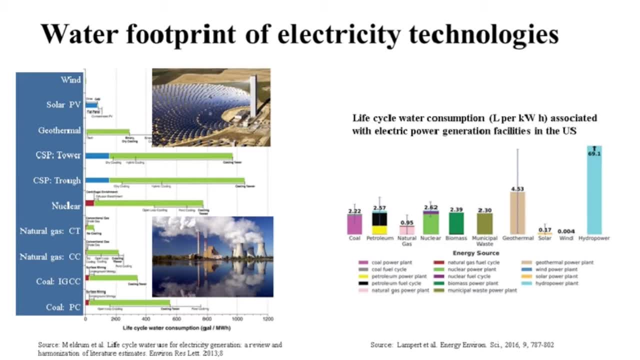 especially during the operational stage, because water is used as a medium to transport heat. by the green bit on the figure And in comparison, PV and wind generally have very low water requirements, especially wind. From the figure on the right you can see that. 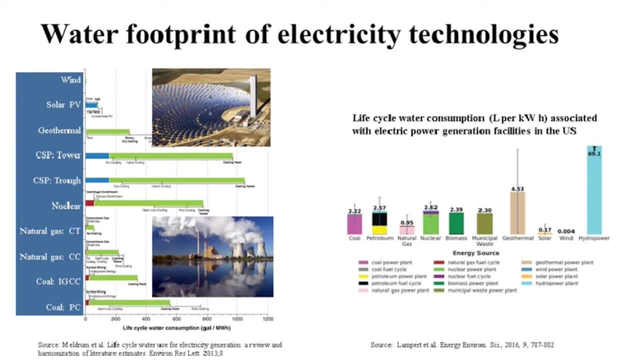 hydropower dwarfs everything else, And that's again mainly because of huge evaporation loss from reservoirs. So understanding these water impacts are critical, particularly for any area that's arid and has limited water resources. Another point I want to make is that the environmental performance 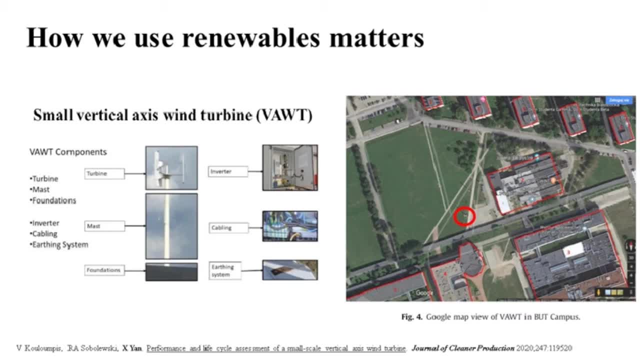 of renewables is not just down to the technologies themselves. How we apply them can also matter. So this is an LCA we did on a seemingly promising renewable technology: vertical-axis wind turbines. Now, these turbines are generally much smaller than the horizontal-axis turbines and do not have 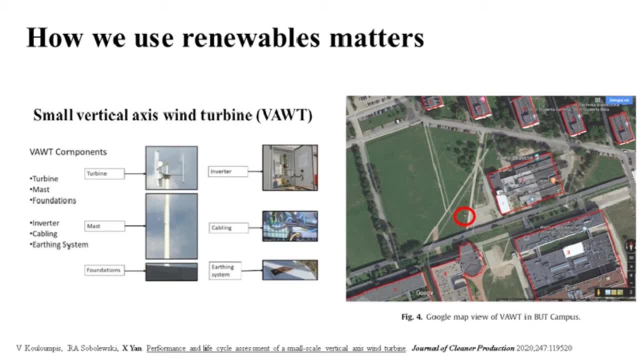 long, sharp blades, So they can be installed in many, many more places, including urban areas or even on top of buildings. So in this study we assessed the impacts of this particular turbine technology, installed at a university campus in Poland, using actual performance data monitored. 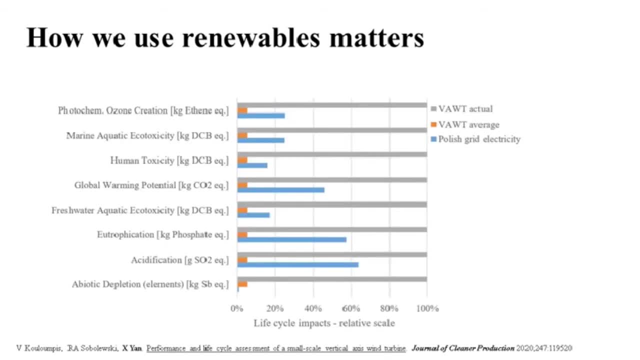 over three years. Now, what we found was pretty shocking. actually, The impacts of electricity generated from this turbine, the gray bars, were much worse than the electricity on the Polish grid, which is dominated by coal power, shown on the graph as the blue bars. 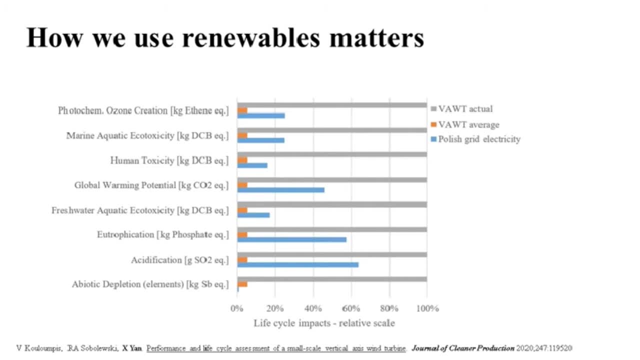 So the gray bars are the impacts of electricity generated from this turbine and the blue bars are the Polish grid electricity, which is dominated by coal power, And the reason for this very poor performance of the. sorry, the reason for this is the very poor performance of the turbine at this. 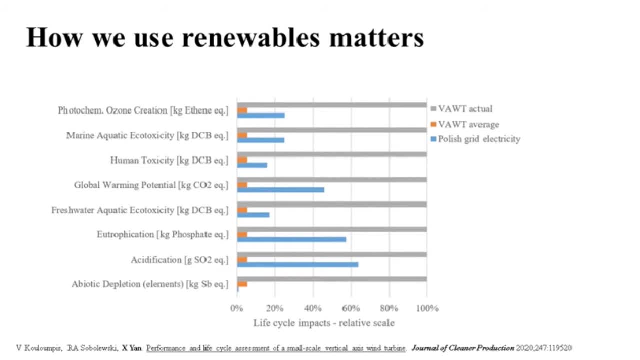 site where it only achieved a capacity factor of 0.5% due to the low wind speed, And the average capacity factor for vertical-axis turbines we found in the literature was 9% And if we use this number, the 9% figure. 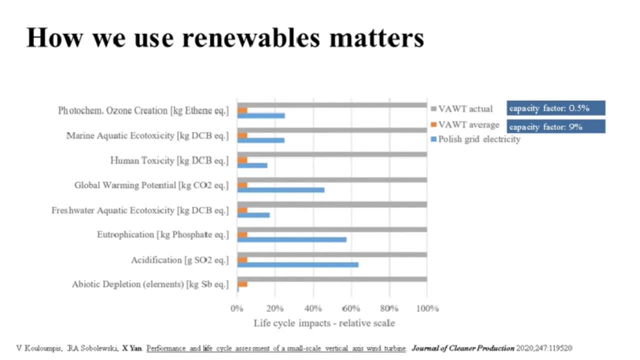 and we put the turbine at a site that has much better wind speed, its impact would reduce drastically. as you can see from the orange bars, They're now lower than the blue bars. Now this is not difficult to understand, as the embedded impacts for the turbine are fixed. 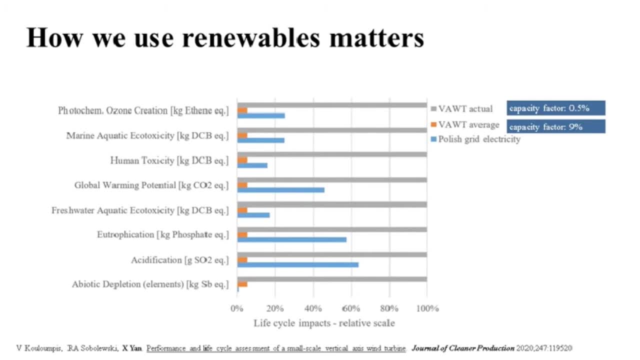 So more electricity it can generate over its lifetime, the lower the impact per energy output. But you can notice that even then there's one particular impact category called abiotic depletion, where the turbine is still worse than coal power, even if we use a 9% capacity factor. 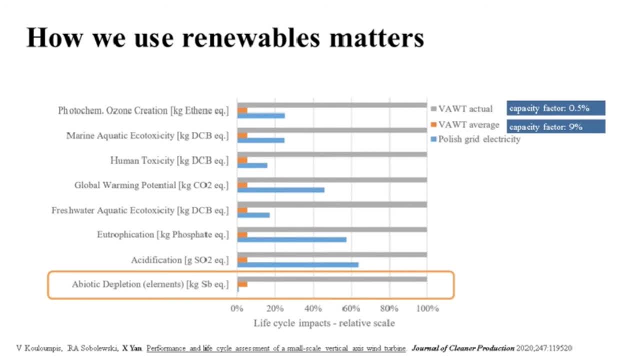 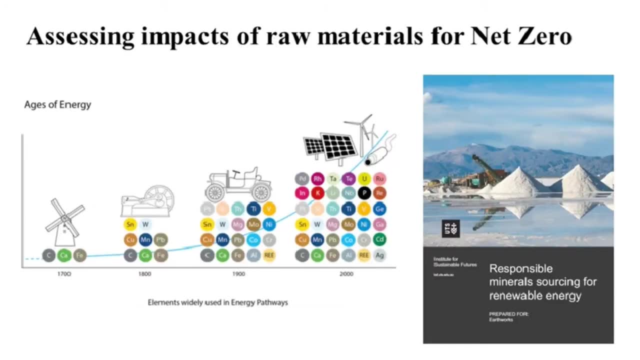 And this is basically due to the higher demand for minerals and metals for renewables compared with fossil fuels, as I mentioned earlier. So this leads to my last topic: sourcing of critical raw materials for low-carbon energy technologies, which is really key to our ability to reach net zero, in my view. 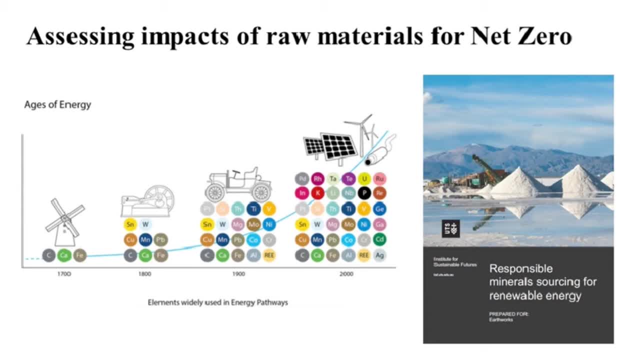 Now. clean energy is an area experiencing exponential growth in terms of innovation and there are so many new technologies emerging these days, But I think we need to be extremely careful because many clean energy tech can potentially have higher impacts than the conventional energy that we use. So I think we need to be extremely careful because many clean energy tech can potentially have higher impacts than the conventional energy that we use. 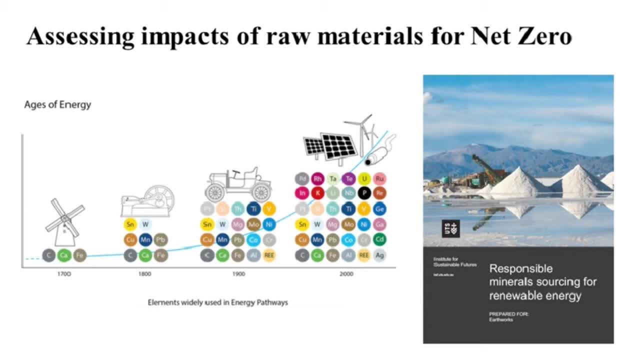 that they aim to replace from a whole-life cycle point of view. Now, the reason for this, or certainly a significant part of the reason for this, is that clean energy tech in general uses more types and larger quantities of raw materials than conventional energy, leading to a rapidly increasing demand for a wide range of metals. 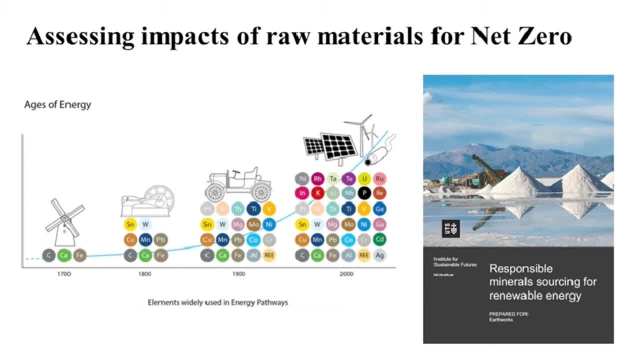 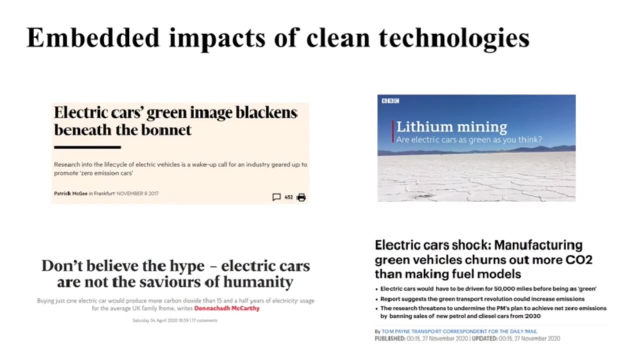 and yet the impacts of extracting, processing and, potentially, recycling of many of these metals, particularly the critical ones such as rare earths, lithium, cobalt, are still poorly understood. Now, the energy and the mining industries are, of course, catching up with this issue, because the consumers and policymakers are now much more aware of these. 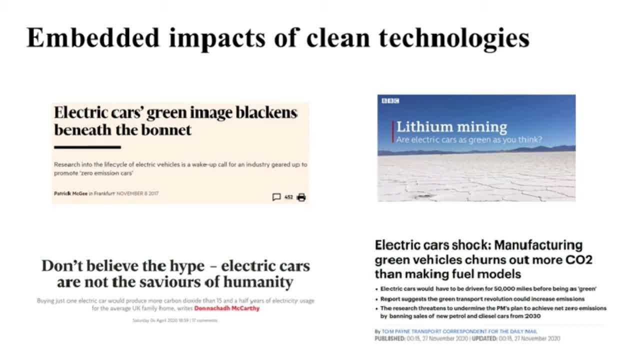 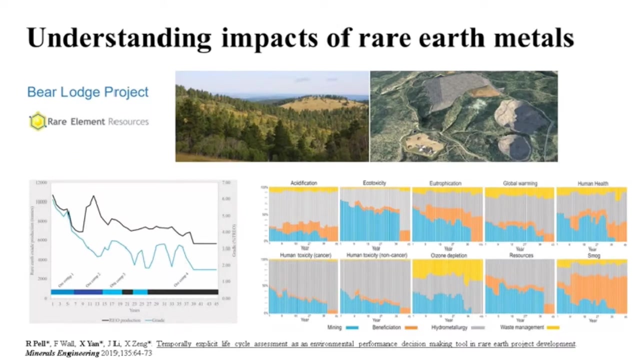 upstream impacts than before And, of course, there's a lot of media attention and also academic debates going on regarding the sustainability of many renewable technologies, low-carbon technologies, such as electric vehicles and hydrogen, And this is why we need to make sure the raw materials that we use in these clean technologies, particularly the most impactful ones. 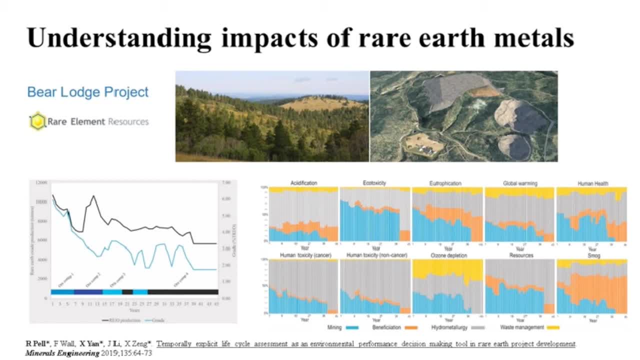 are. the materials that we use in these clean technologies. particularly the most impactful ones, such as rare earths, are produced environmentally responsibly, And we've done quite a lot of work helping mining companies to understand and improve their environmental performance. For example, a former PhD student of mine used LCA to assess the impacts of rare earth elements. 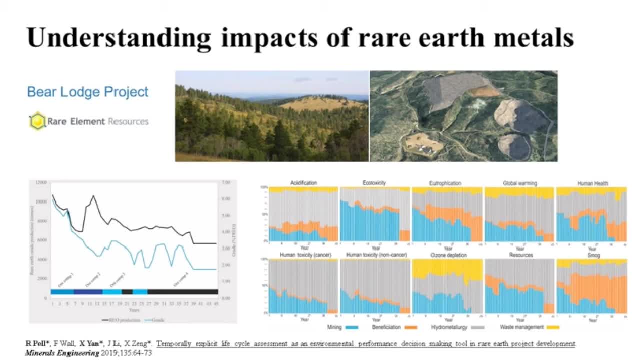 What's shown here is an example, And during his PhD he developed a number of modeling techniques and metrics and data sets specific for minerals and metals, which turned out to be quite valuable And in fact, there was so much demand for these tools and data from the mining industry. 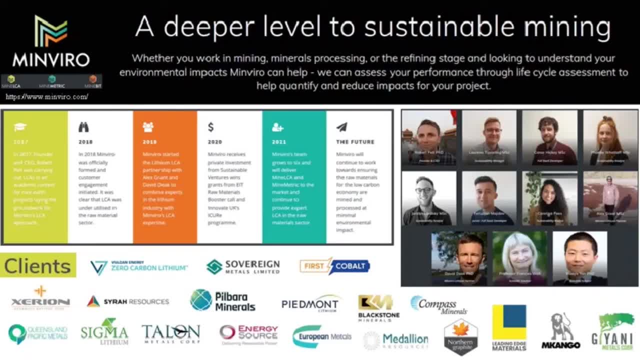 but also the investors community, that he decided to set up a spin-out company called MinViral to commercialize the IP, And we've successfully secured private investments and innovative UK funding to scale up consultancy activities and further develop our proprietary software tools and databases. Over the last year alone, we've already worked with more than a dozen. 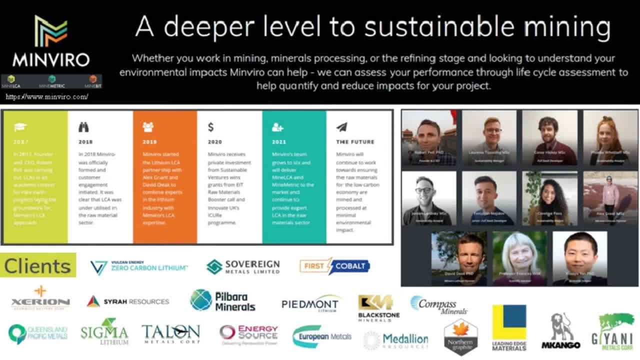 mining companies to help them improve the environmental performance of a wide range of minerals and metals for clean tech, such as lithium, cobalt, nickel, magnesium, graphite, in addition to rare earths, all of which are very important for the environment. 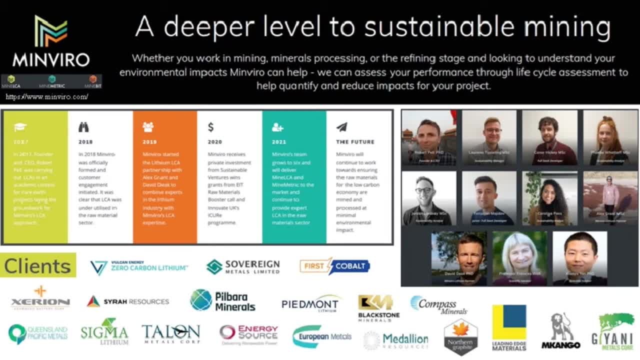 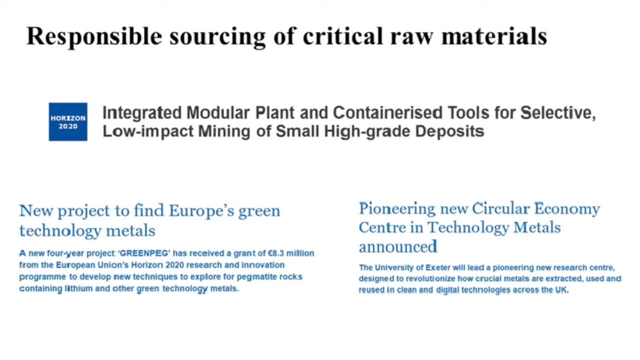 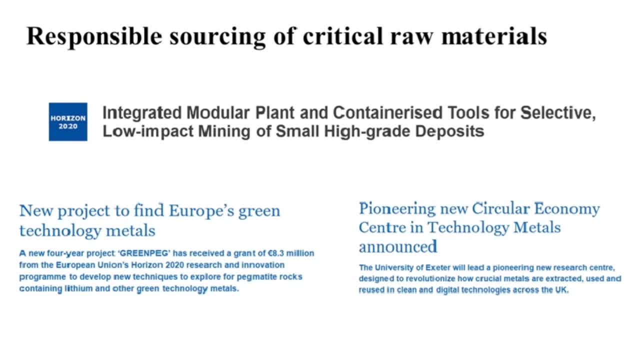 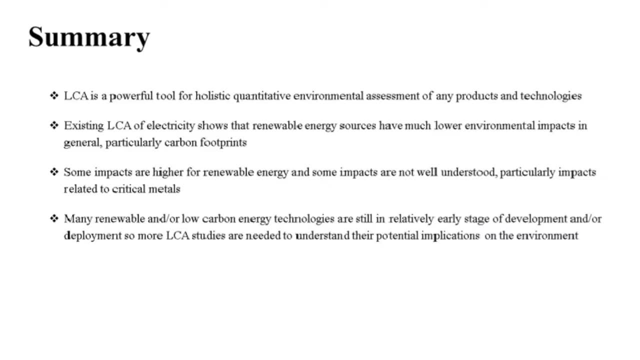 And we also believe that the potential cumulative impacts of a significant increase in mining activities driven by clean energy adoption have so far been overlooked. Finally, a quick sort of summary of what we talked about. LCA is really a useful tool for assessing the environmental impacts of any products and technologies. Existing LCAs on electricity. 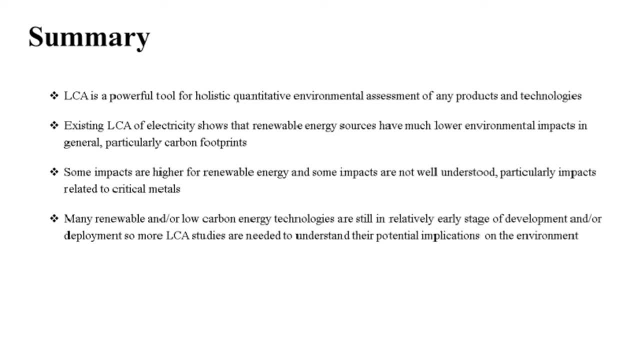 generation show that renewables generally have much higher energy efficiency than other technologies, with much lower environmental impacts- carbon footprint in particular- than fossil fuels. But there are impacts where renewables can perform worse, such as land occupation, and there are impacts that are not well understood, particularly ones related to critical metal production And 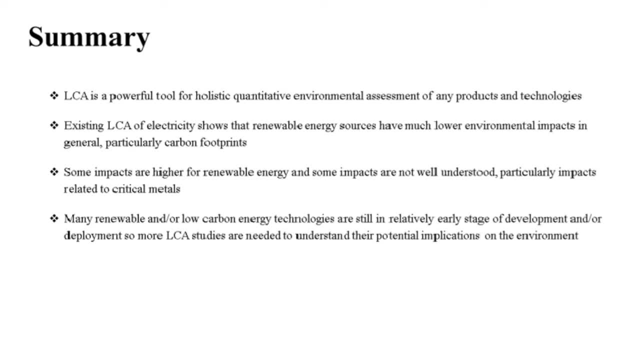 given that many new technologies are emerging in the renewable or low carbon energy space, we need to use LCA to understand their potential environmental implications in order to make sure that they are truly sustainable in the long run. And that's the end of my talk. 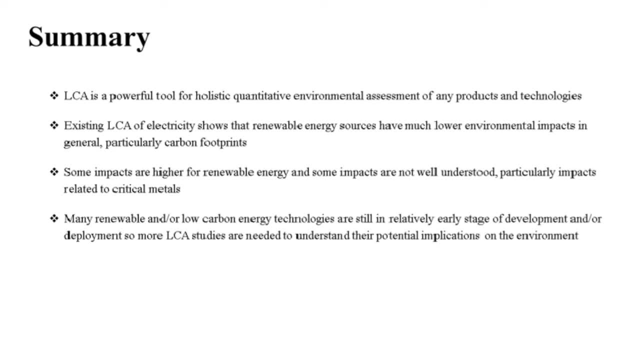 Thank you very much for your attention and I'm happy to answer any questions you might have. Thank you, Thank you for that. That was, I think I'm sure we'll all agree, an excellent presentation on a really important topic that is only going to become more important. 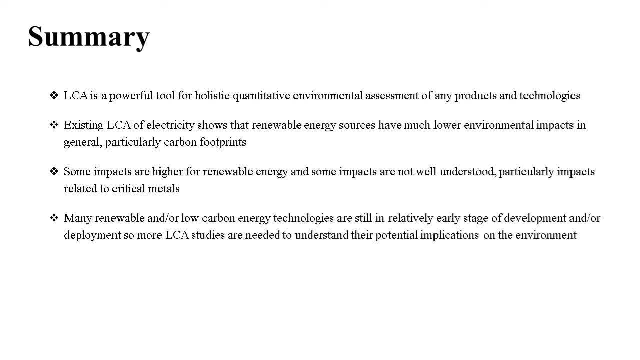 as we go forward, and it's good to see that there's some really, I think, useful work going on there at the University of Exeter, in the Environment and Sustainability Institute, where HU works. We also have now a lecture from Professor Richard Cochrane Just before that. 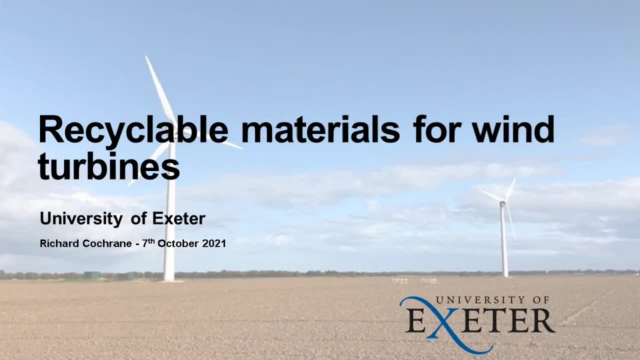 I'll just add in that there is the opportunity. if you have questions, you can type them into the Ask a Question chat bar and we'll do our best to come on to those and have some time for discussion at the end. I'll now hand over to Professor Richard Cochrane, who lectures also at the University. 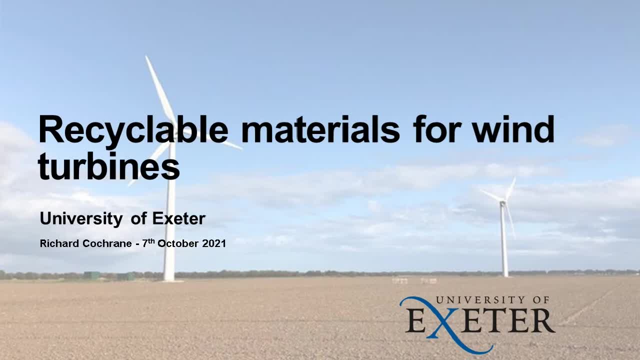 of Exeter and the campus in beautiful Cornwall, and Richard will talk to us about recyclable materials for winter pines. Great, Good afternoon everybody. I hope you can all hear me, okay. Thank you for talking to our youth. As I said, my name is Professor Richard Cochrane. 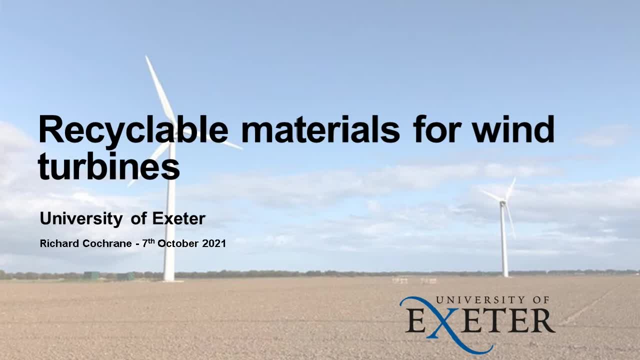 I work with the renewable energy group based at the University of Exeter down in Cornwall. We've got a team working on offshore renewables, looking at wave and tidal power and actually recently increasingly work on offshore wind and particularly floating offshore wind as the next. 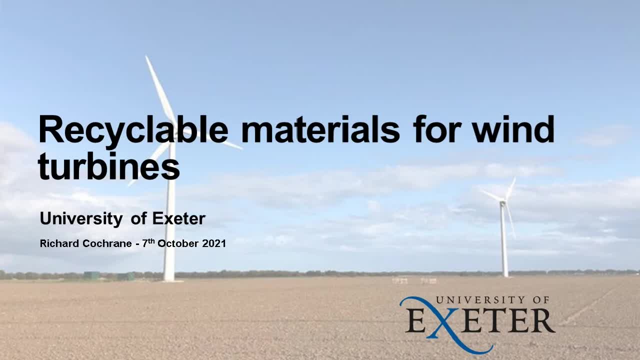 development in that sector. We've got a group working on the latest solar technology, the next generation of solar panels, and then supporting work, Zhao Yu on the lifecycle analysis, colleagues who work on the connections of renewable energy systems to the grid. 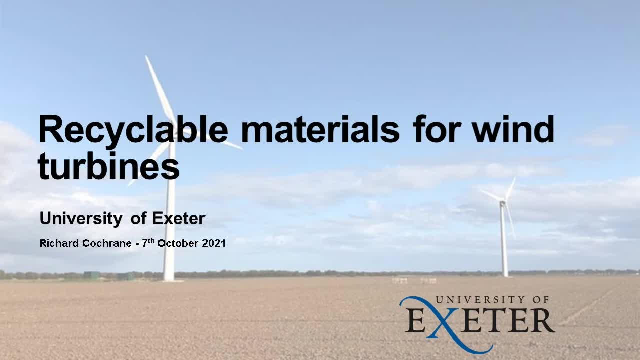 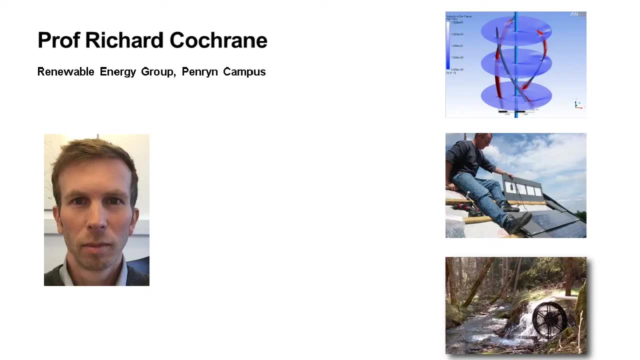 or the connection of energy storage to the grid, as well as work on energy storage technologies and the policy framework that renewable energy is deployed within. Personally for me, my background is was starting off in general engineering and I've been working in the industry for a number of years now. I've been working in the 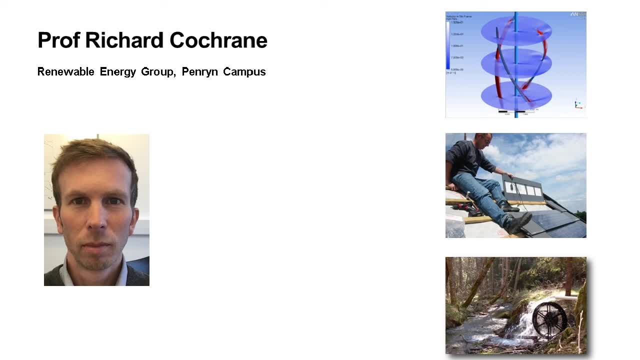 industry for a number of years now. I've been working in the industry for a number of years now, So we've worked on energy and buildings, looking at energy efficiency, but also integration of renewables, developed products like the solar tiles to try and facilitate easy installation of. 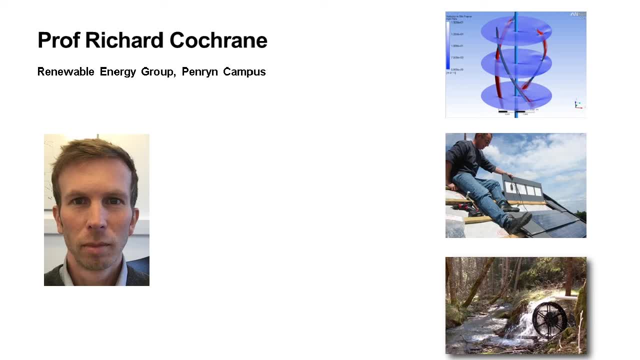 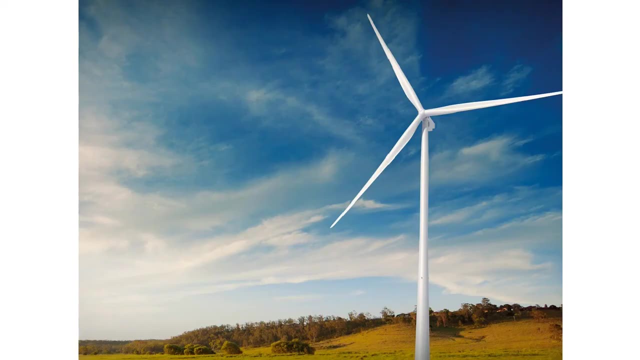 solar with existing building stock. We've developed a vertical axis wind turbine- the helical form- to work in turbulent wind environments, and I've worked on hydropower And other technologies like that. In terms of wind, the focus today, I have really been, I suppose, very impressed with the progress that we've made. 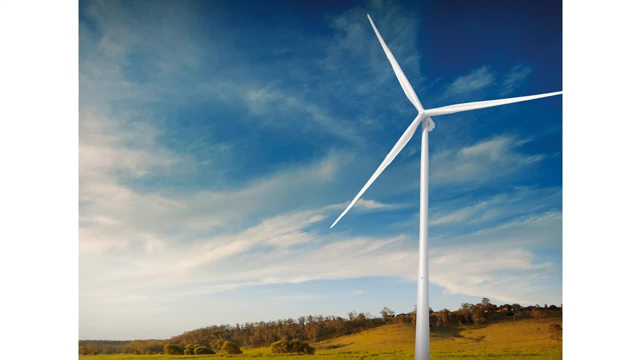 in the wind energy sector. Very exciting that the sector is now cost effective. We always used to have to push. we were pushing for renewables but had to fight for subsidies or other financial support because it was more expensive. But 2015 onshore wind became cost effective without any subsidy. It's cheaper to make electricity from. 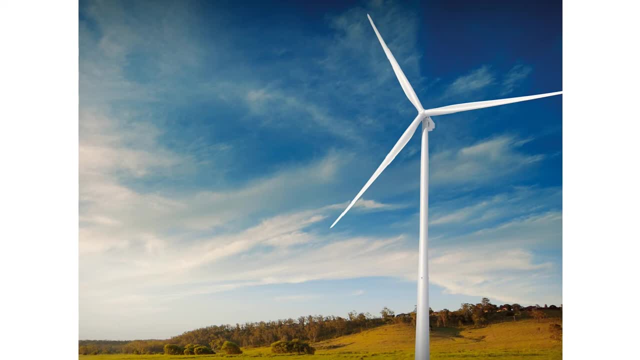 wind than it is from fossil fuel technology, which has been a very exciting crossover point on that. Now the technology really has come on Externally. perhaps a modern turbine looks rather similar to technologies that were put up 20 years ago, but they perform so much better. 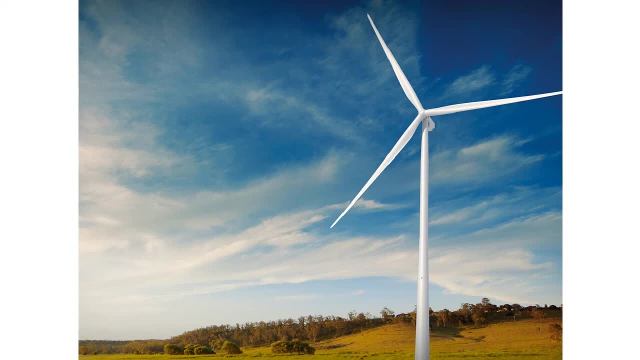 We recently visited Goodehilly Wind Farm, the second wind farm that was developed in the UK And on that site used to have 14 turbines And it was repowered with six modern units. Now those six turbines generate three times as much energy as the 14 old ones used to, And 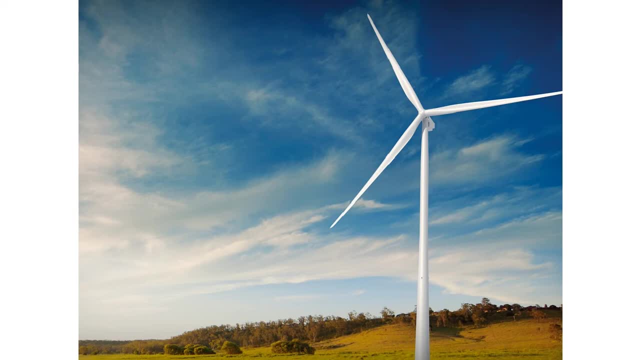 as well as that, they are considerably quieter Because they're larger, they turn more slowly, So I think they're rather more graceful. There is a challenge: that they can be seen from much further, because they are taller, So you can see them from further apart. But actually 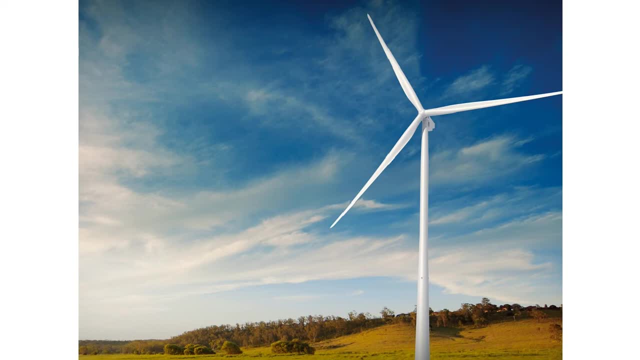 local residents were concerned about that repowering with these big machines coming in. But actually now they're in, they see how much better they perform, how much quieter they are, how graceful they are And they're delighted with them. They basically make that area carbon neutral from the energy that's involved in them. So onshore wind has been. 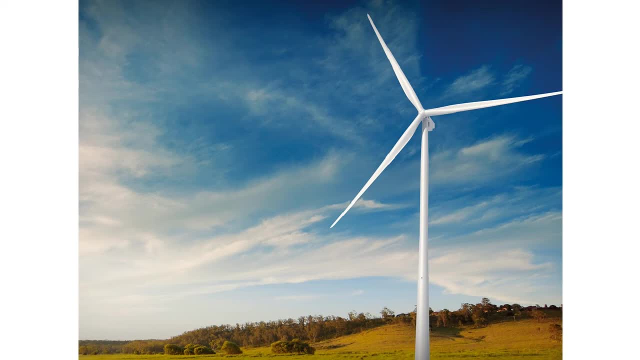 very exciting In those days. they've been in the wind farm for about five to six years, So, but there is a challenge: that they can be seen from much further because they are taller. so you can see those sort of developments and increasingly we're seeing real progress. 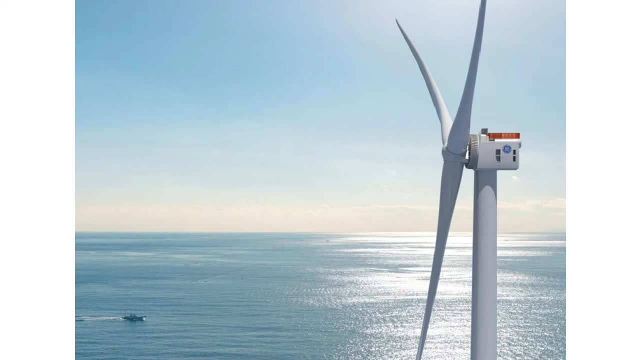 in the offshore wind sector. A little while ago there was the government plans to highlight that we're going to deliver about 40 gigawatts by 2030 of combined onshore and offshore wind and, like onshore wind, again very exciting- that offshore wind is now viable effectively without subsidy. It's still supported by 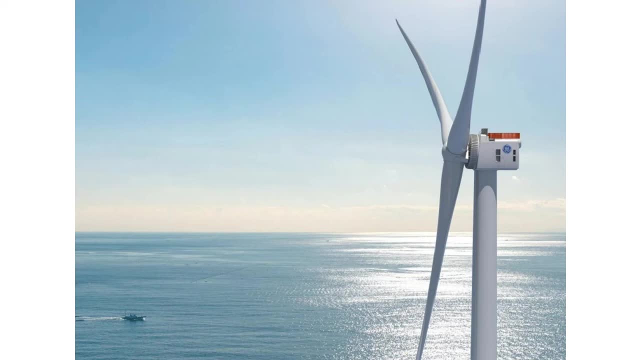 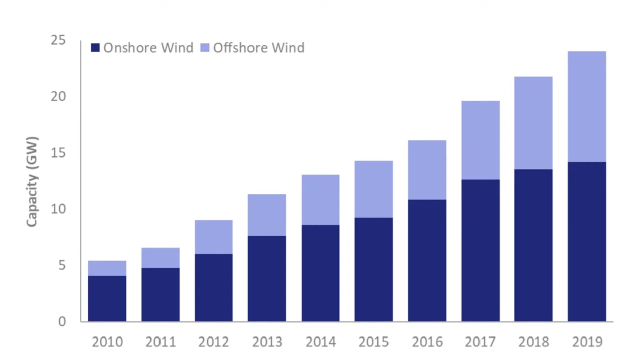 the CFD contracts for difference, but they agreed a price which is effectively lower than the pool price of electricity. so, in effect, wind, offshore wind- is now viable without a subsidy going forward. So we've seen good, steady growth in the wind sector and there is still. 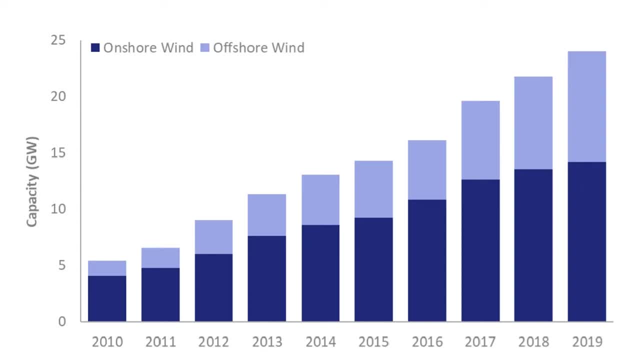 quite a bit of growth in the offshore wind sector. Onshore wind being deployed in perhaps less in England but more in Scotland, Wales, due to planning arrangements. but particularly the growth we're seeing is the offshore wind sector. Now what does that do overall? These are the latest. 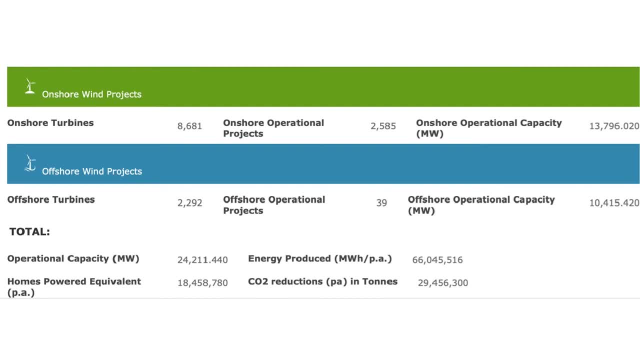 figures from Renewable UK who support the industry and highlight the sort of 24 gigawatts of total installed capacity that we have. and I quite like the figure that actually those turbines generate as much electricity every year as is consumed by eighteen and a half million homes, so really quite a good. 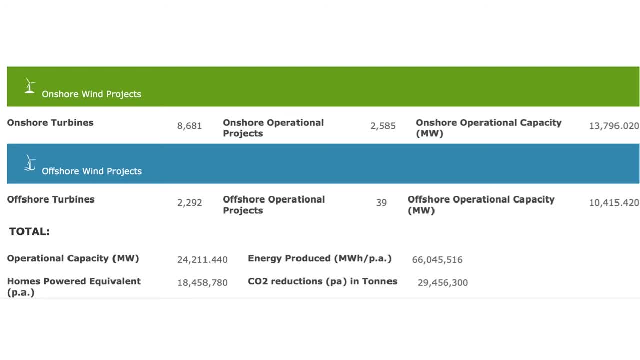 contribution to our energy network and it's- I've been very impressed with how that's worked- to decarbonize the electricity that we generate. Six years ago- typical values eight years ago perhaps the carbon intensity of our grid was over five hundred grams in for every kilowatt hour consumed in electricity and typically now that's. 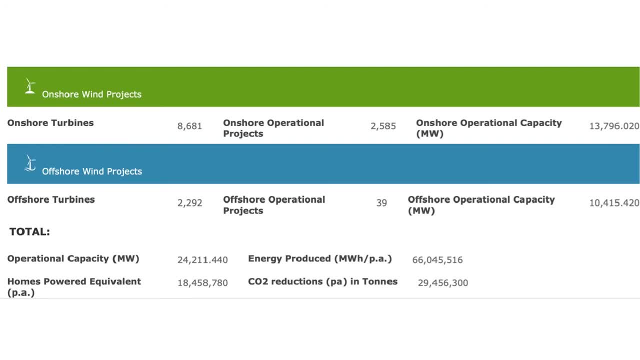 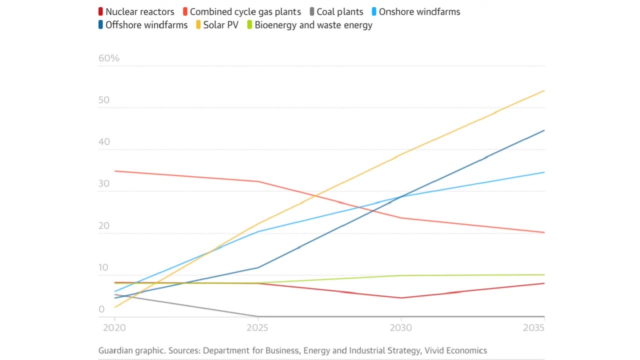 about 200. I just looked at the figures- you can- it's all available on the web- and today is about 230, and a quarter of our power today is coming from wind energy in the UK, so that growth is forecast to continue. you can see the blue lines here: onshore and offshore wind, both forecasted considerably grow. 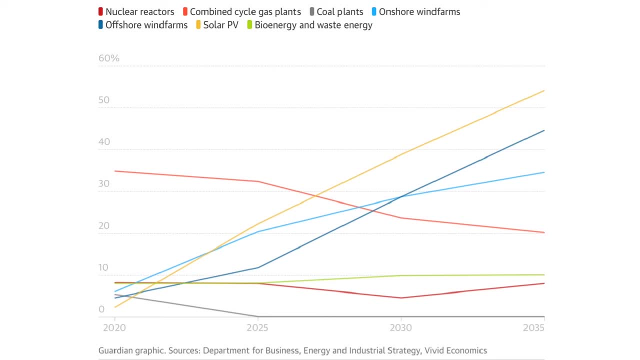 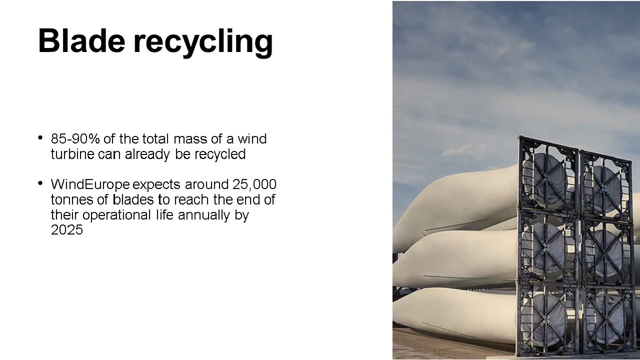 and an increasing contribution to our energy performance going forward. but we are finding from that, particularly the early deployment, that the first generation of turbines are coming to the end of their. you know, the first generation of turbines are coming to the end of their nominal design life and the industry is working hard to work out what to do with. 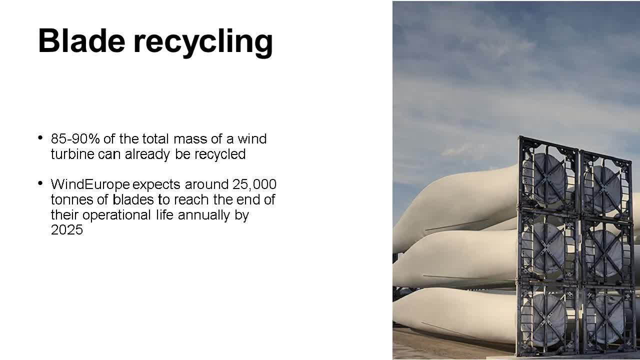 them now to put some context around. I think the blades are the area of focus that will will explore further. but overall, actually, the majority of the mass of a wind turbine can be relatively easily recycled. the bulk of the weight of a turbine is the tower, the structure around the nacelle, the gearbox, the 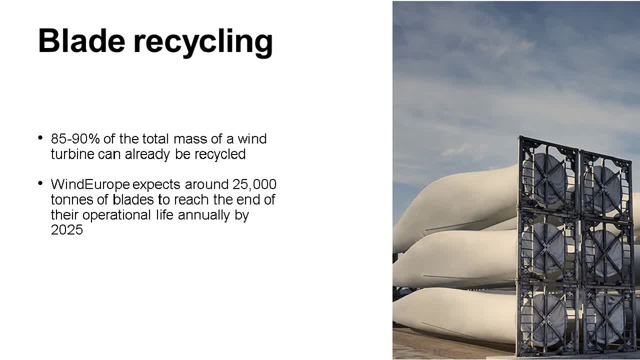 generator and those metal steel components can be recycled quite easily. 85 to 90 percent of the total mass can already be recycled quite easily, but we are looking at potentially still 25,000 tons of blades that will reach the end of their nominal life within the next few years. now these blades have been designed for for long-term use. 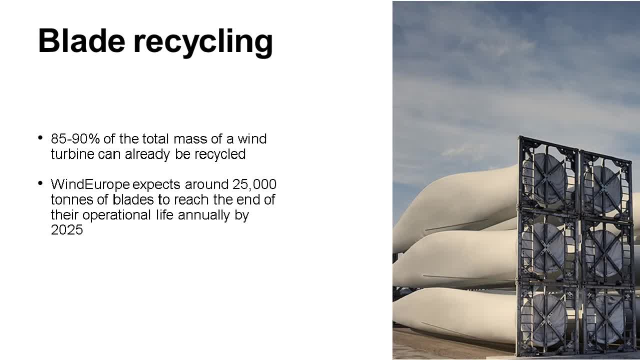 Now these blades have been designed for for long-term use. They've had the longevity to be out in the environment for years, decades, and they work very well. but when they were designed, recycling was not, unfortunately, the priority with the design life. they were designed to materials available at the time and that's. 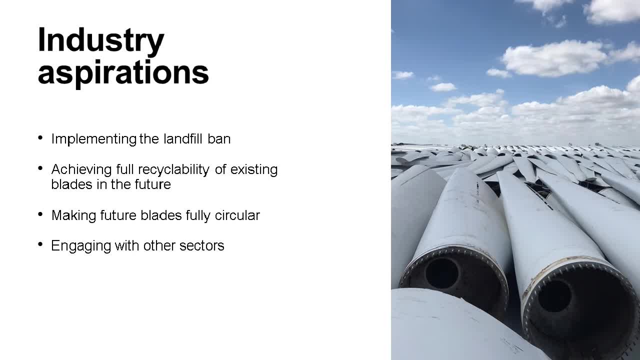 yeah, they are hard to to recycle. Now industry fully recognizes this- the challenges of the waste of all these blades and are keen to avoid them going into the landfill- are looking at ways to increase the recyclability of blades in the future. looking at the sort of full 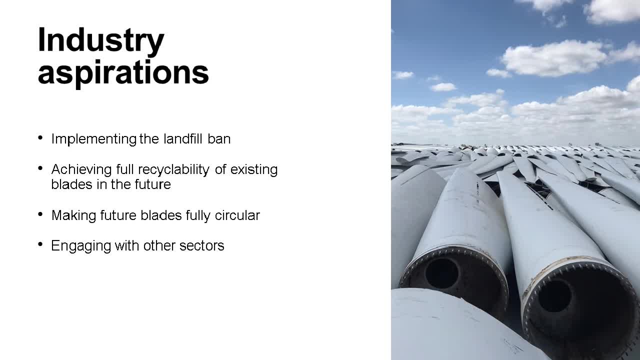 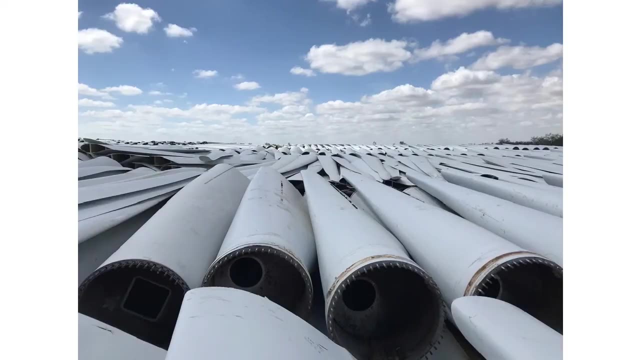 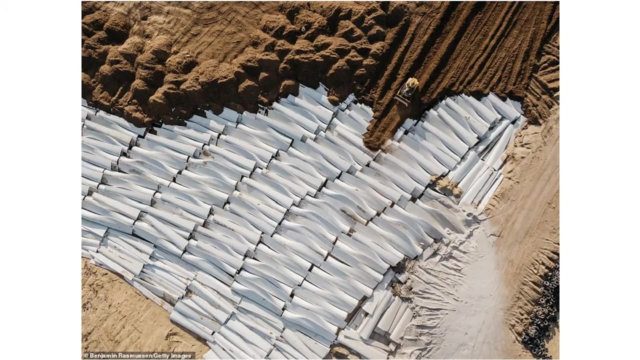 circular economy, understanding the whole lifecycle of the blades and what can be done with those materials at the end of their life. so it is an issue you what's going to happen with these materials? And there have been cases where, like this image here, blades have been, because there wasn't a process available at the time, chucked into. 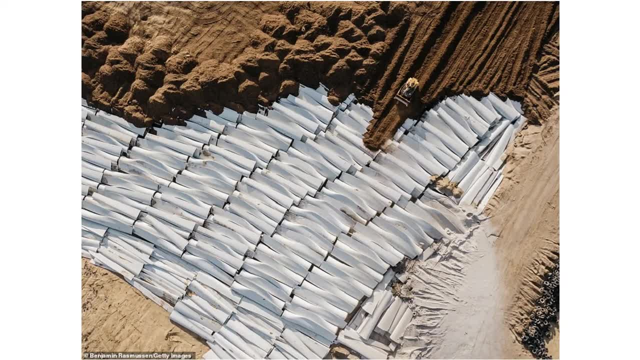 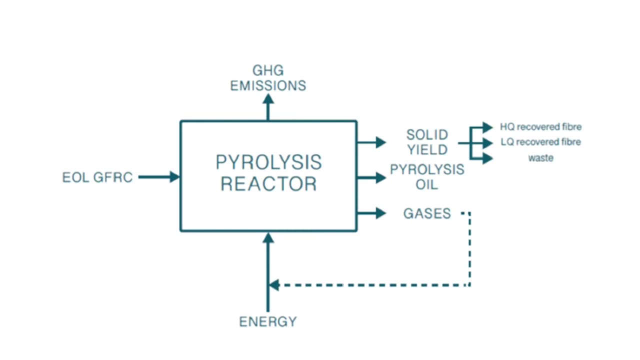 landfill, which is really not an appropriate solution for this, If they are simply being disposed of. there are technologies that are being explored that could be far better in terms of the energy consumption. One of those is pyrolysis of the blades, which is a route to recover some of 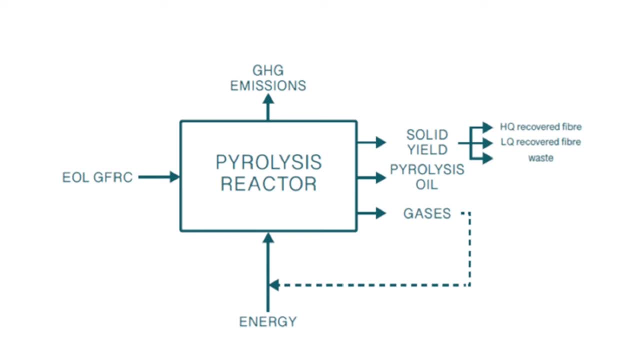 the material involved in the blades. So this is almost like melting the blade- super high temperature but with very limited oxygen supply, And it breaks down the components relatively effectively. It is possible to recover some of the fiber, the glass fiber and things from the blade materials. 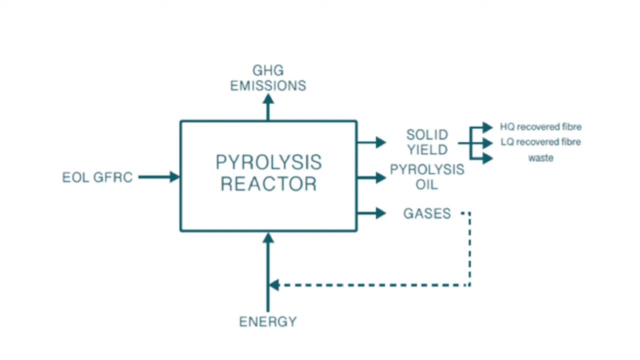 which could be reused, And then the pyrolysis oil that comes off has a variety of options that it could be used for in terms of plastic manufacture or other things like that. It could be burnt, but then that's releasing carbon dioxide into the atmosphere, which is what we're trying to. 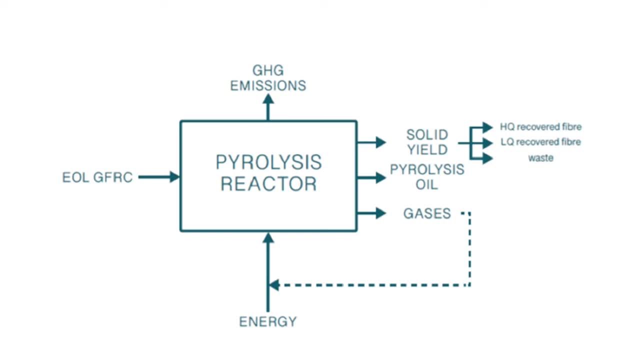 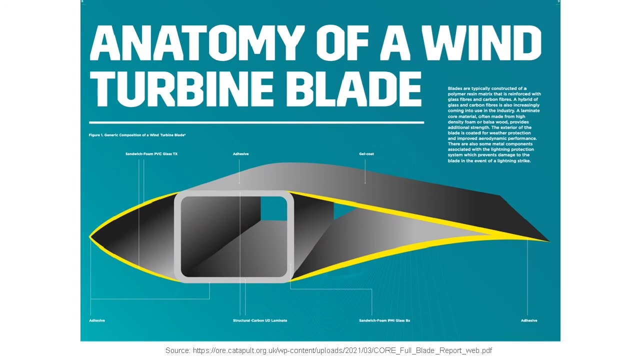 avoid in a sense. So it isn't in a way quite straightforward what to do with the blades. Externally a white lump of plastic, but actually internally, really quite involved composite structures. They work and have a phenomenal loading on them from the wind And you have a sort of box section illustrated here. 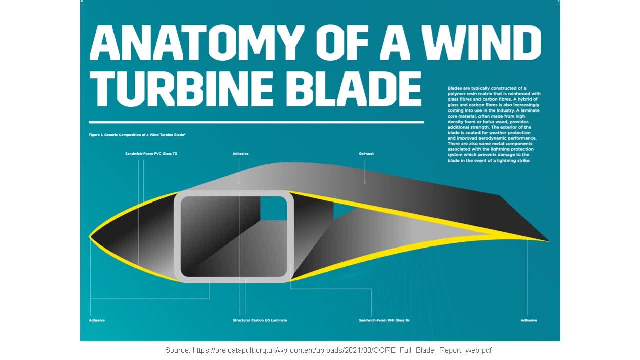 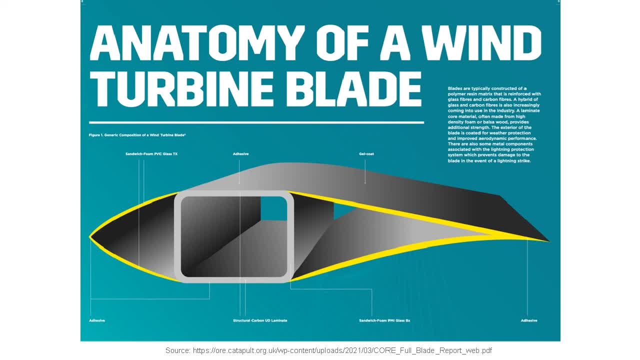 And that's what sort of minimize: the more expensive carbon fiber, just where it's doing the most work structurally. But the other parts of the blade to create the airfoil shape are often glass fiber, And then there's various filler and other components in there. So it isn't a simple. 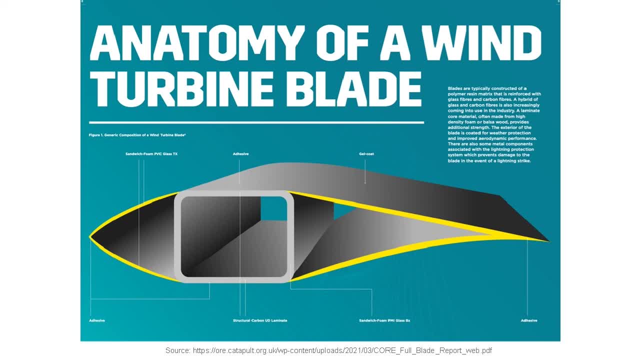 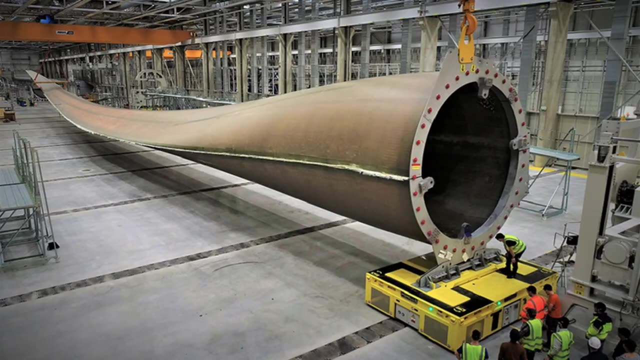 sort of individual bit of glass fiber. It's quite a complex structure. Other elements in it like and then lightening conductor and those parameters which also need to be separated, And we have made really phenomenal progress in actually the manufacturing of these blades- Some of the latest ones are 107 meters long- and developments things like vacuum and resin. 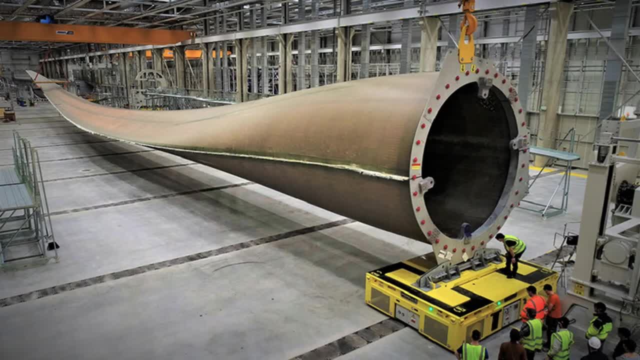 infusion, where, rather than making the blade out of lots of different components and then gluing them all together, some of these latest blades are manufactured in the late milliseconds, I guess, are manufactured in a single process where the internal structure is supported and then dry fibers laid up into all of that molds. 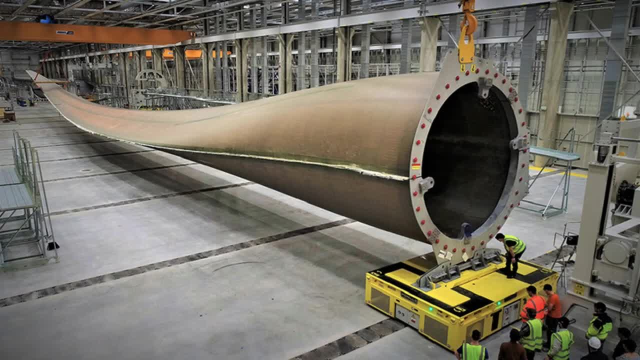 And then resin infusion sucks through an epoxy resin through the whole 107 meter long blades, which has been fantastic in terms of their performance, Because they're all effectively fused in one process. they're far stronger and far lighter, which is very important for the waste loading. 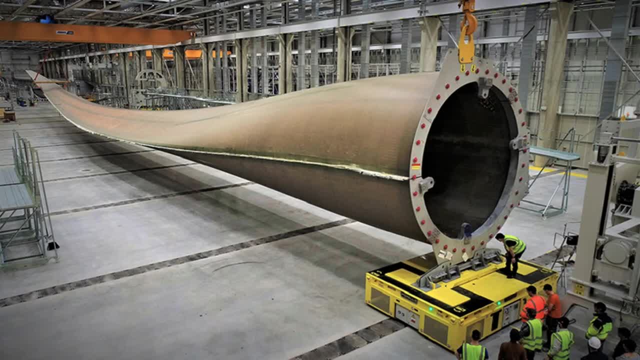 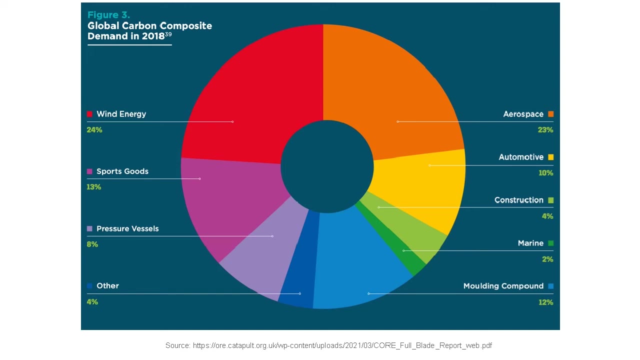 as these blades spin round, It increases their longevity, makes them far more robust and far cheaper to manufacturer relative to their size. And I suppose, just to put the sort of context that said, the industry is also looking at other, collaborating with other sectors, and wind energy is a significant proportion. 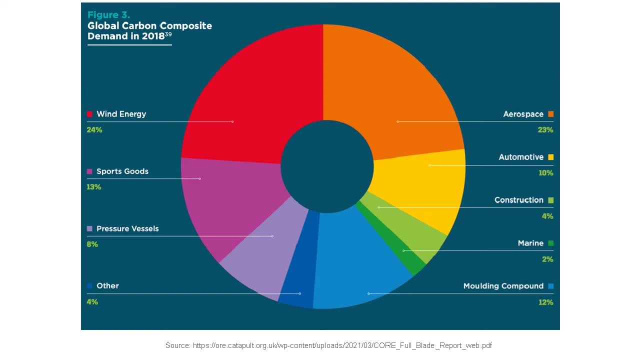 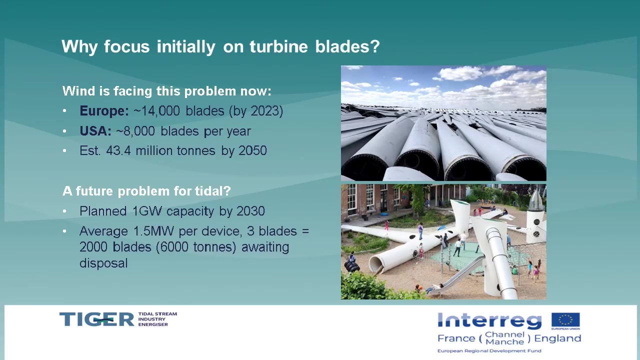 of the composite market, But only just under a quarter of it overall to the aerospace sector, marine sector, construction. all those other areas are also using composites and also need to address opportunities for recyclability of these materials going forward. So I borrowed a few slides from a colleague who's been looking. 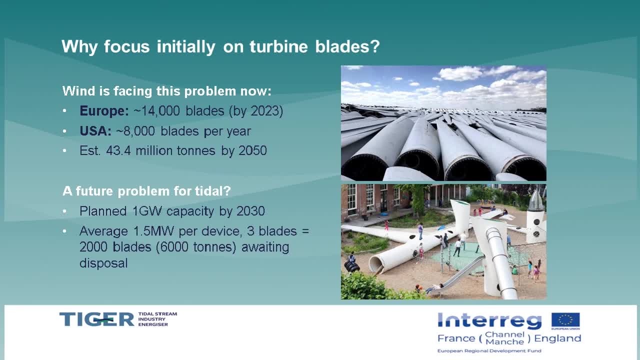 at this area, but particularly focused on tidal technology. So thank you, Stuart Walker, for these images summarizing some of the work for this. the entire project looking at tidal, in innovations in tidal energy Highlights again those: the number of blades. 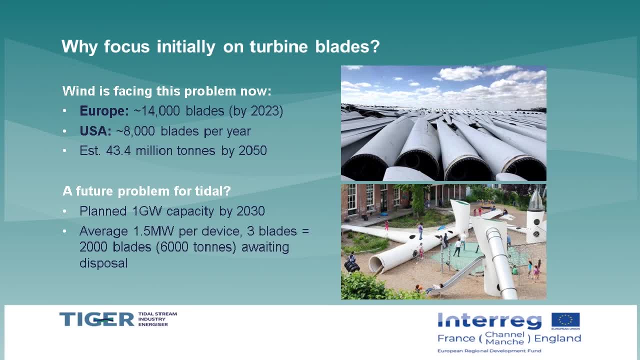 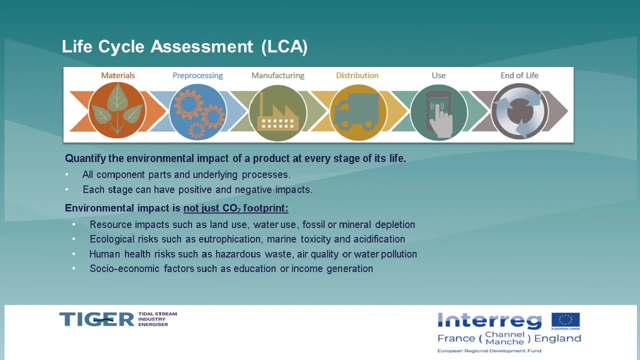 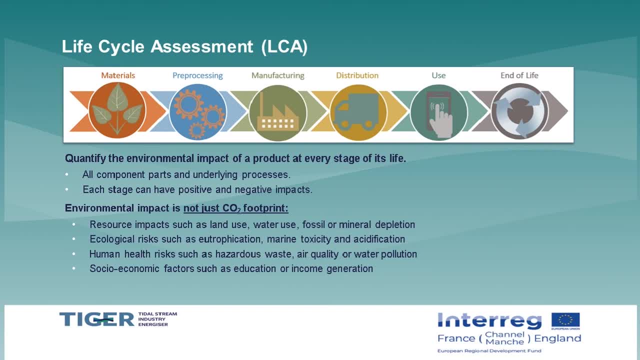 So, as you highlighted, it's very important to consider the full life cycle analysis of this and not just focus on the performance and energy optimization at this stage. Overall, I've been very impressed. I think a large wind turbine does use energy in its manufacturer, but it generates so much energy once. 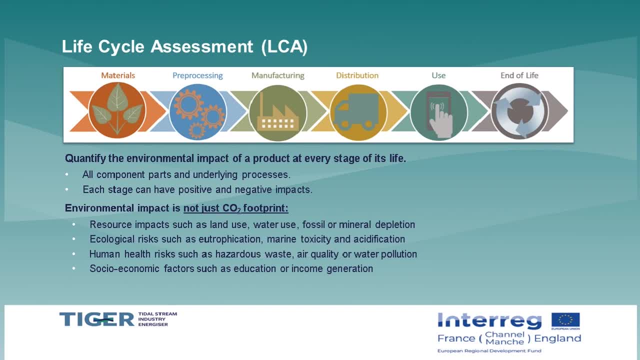 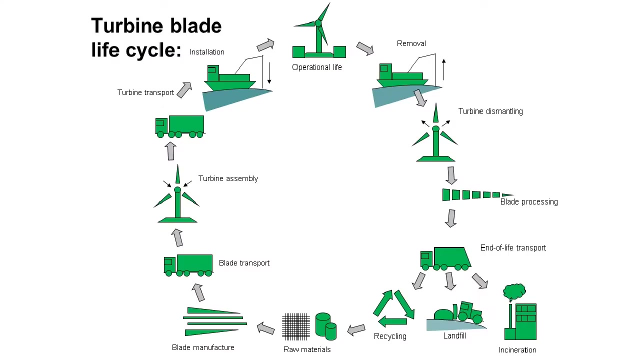 it's in operation that within six to nine months it has saved as much energy as was used in the construction of that solar wind turbine, which I think is very impressive, shows remarkable efficiency of the modern units going forward. So if we look at the that full process, 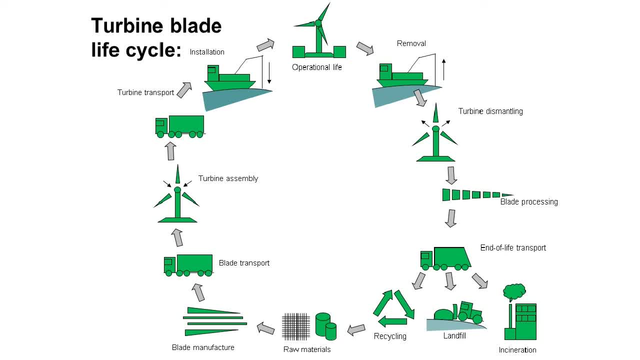 again, as I highlighted, very important to consider the full operational life, what happens at the end of life and then whether that is unfortunately some of them being incinerated, some of them going to landfill, or opportunities to recycle and separate those materials going forward. 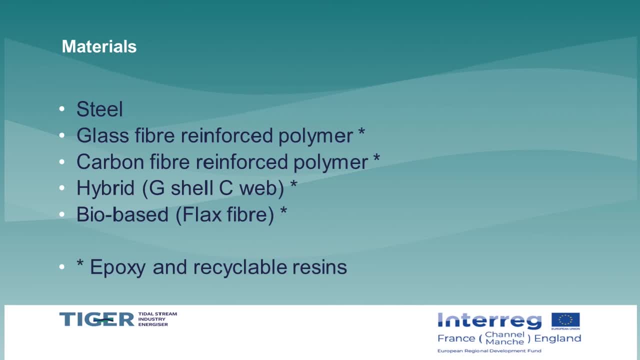 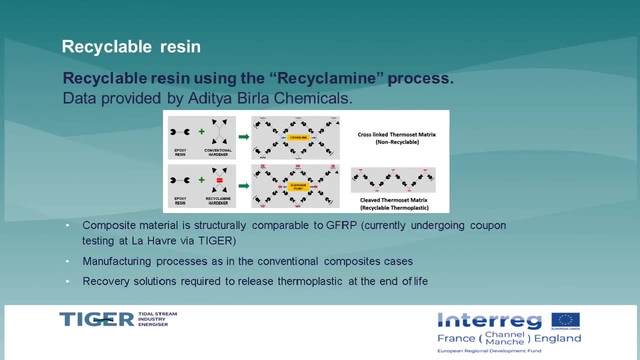 So we do have different materials within that. those structures steel relatively easy, but the real challenge is a lot of the composite materials, the materials that we're working with, And there is real progress in some of these areas At the moment. a lot of the blades were made with a resin. 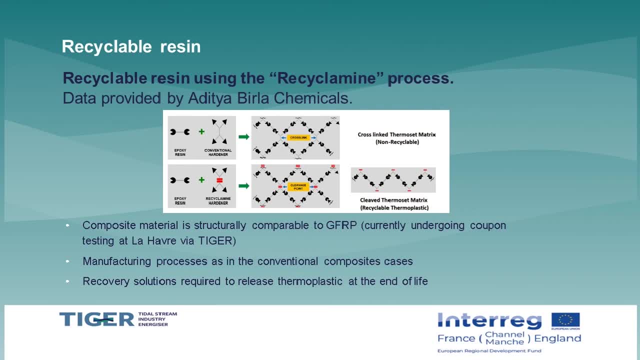 that isn't possible easily to separate from the carbon or glass fibers, but there are companies developing a recyclable epoxy. We did some work to analyze this, thinking well, what's going to be the compromise? This new material isn't going to perform as well. 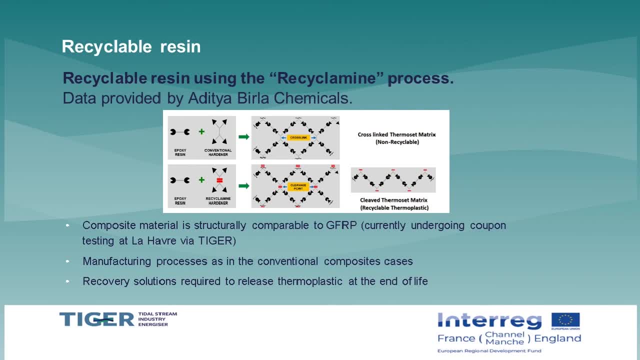 So the material is going to be weakened, The blades are therefore going to be heavier And actually, through all that analysis we found that the blade performance was just as good as the existing epoxy resins and enabled performance with the same strength and weight performance going forward. 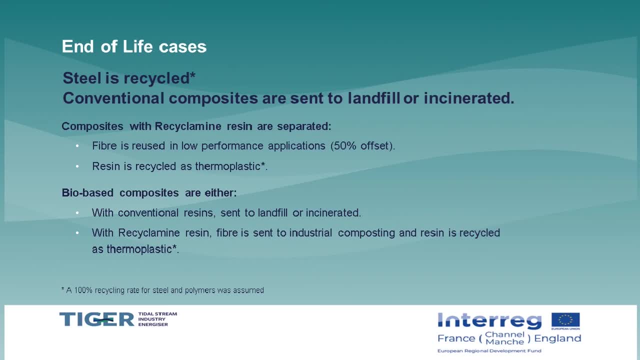 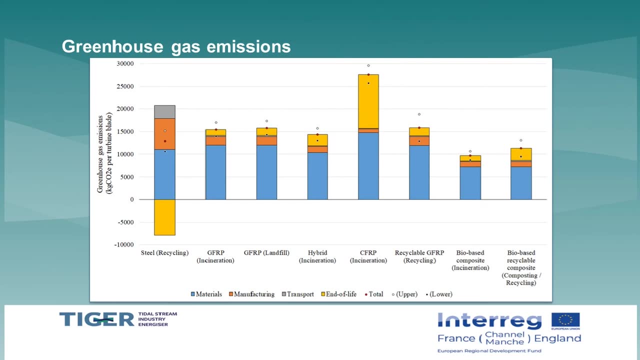 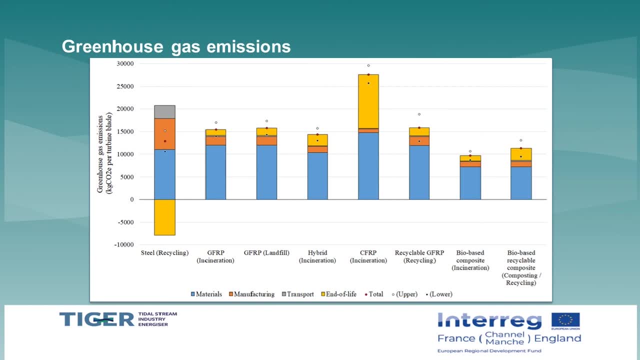 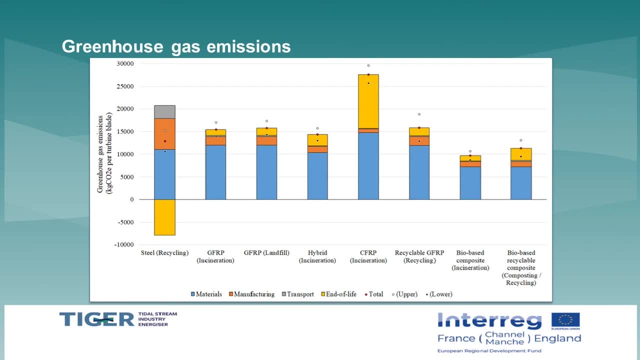 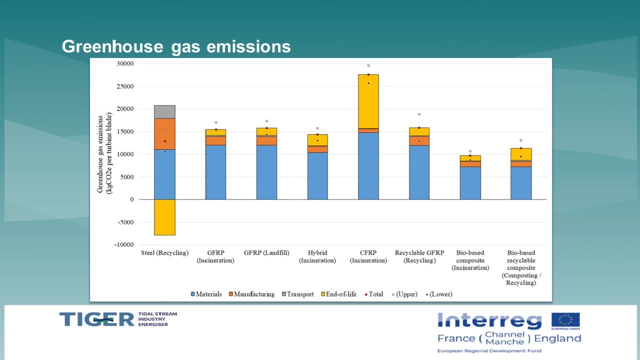 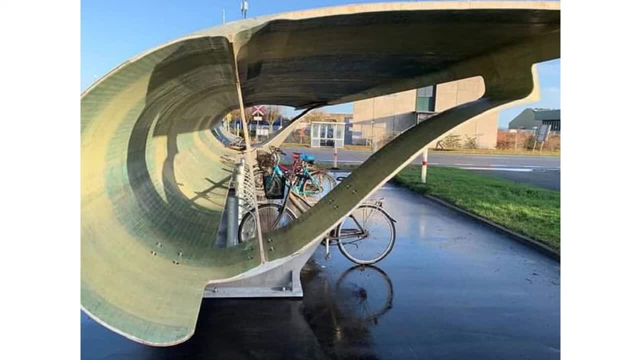 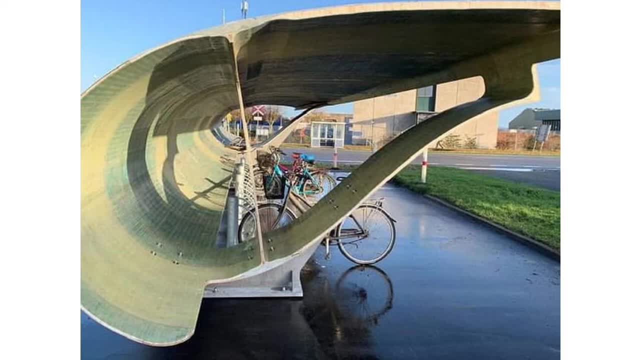 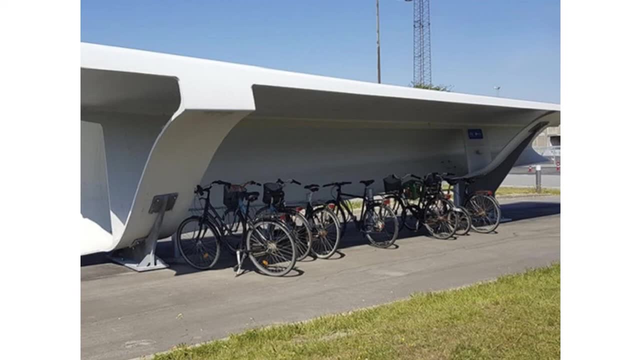 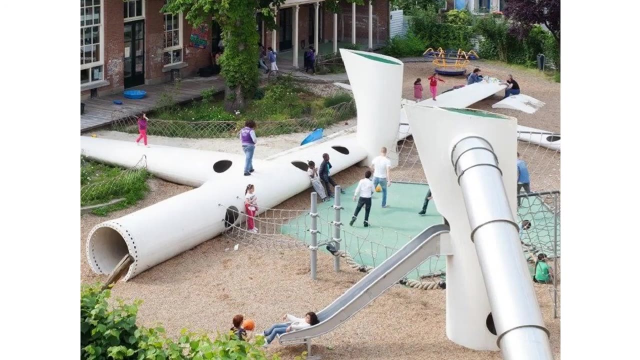 Give it a. I think Nic, Nic, No, No, studied He 초 in holland or denmark. sorry um great opportunity. there then, some very nice examples of, in this case, a child's play area: great fun. i think i've seen some nice examples here where the kids can. 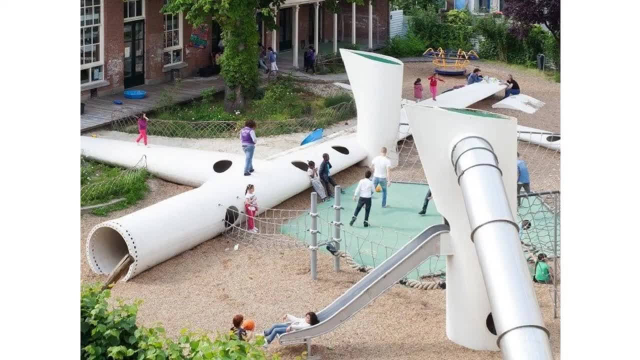 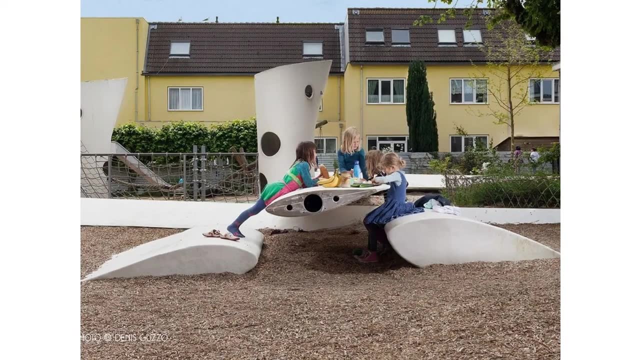 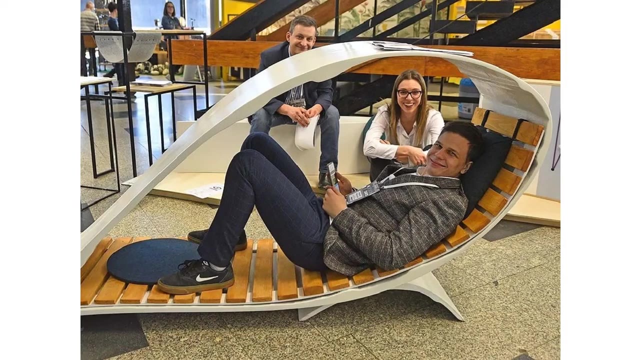 crawl through the tunnel, go up and slide down the slide, and other examples where they've been turned into a climbing wall. um so a nice again further purpose of that. and then innovation in terms of this case, a seating, turn it into a seat, and other opportunities like that. 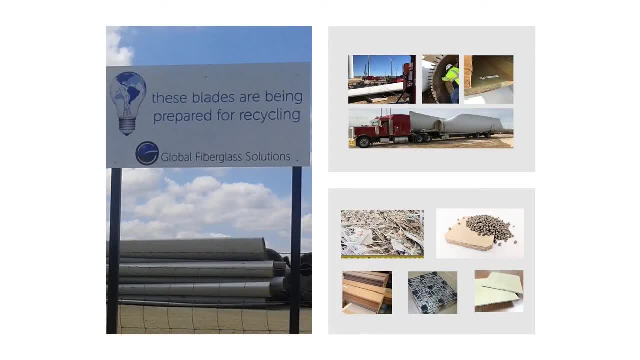 then in other ways there are other opportunities. so this company are proposing almost sort of grinding up the the blades and then creating pellets which are then fused into other building materials. so it repurposes the fiber reinforcement mostly for their proposals into construction materials. so they're making 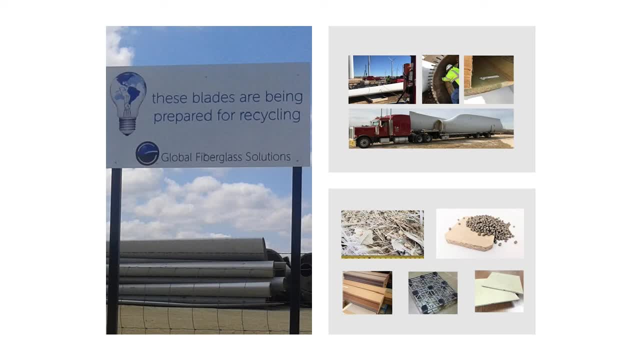 construction panels for buildings that give that the blade life, a second life going forward. so that's a really good example of what we're looking at here. so that's a really good example of what we're looking at here. so thank you very much for that. i. 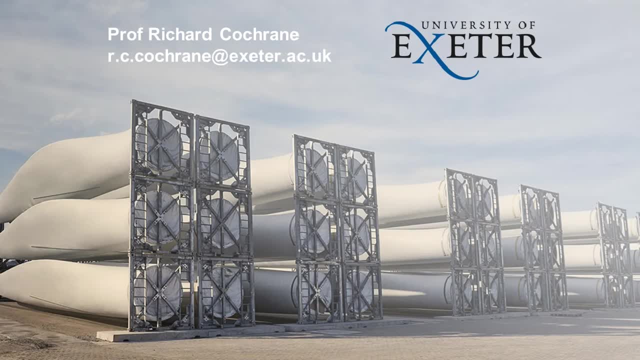 now welcome any any questions on any of those subjects. thank you, hi everyone. it's fiona from the imechi um david is just experiencing some microphone issues, so please bear with us for a few minutes and he'll be back shortly with the q? a. thank you. 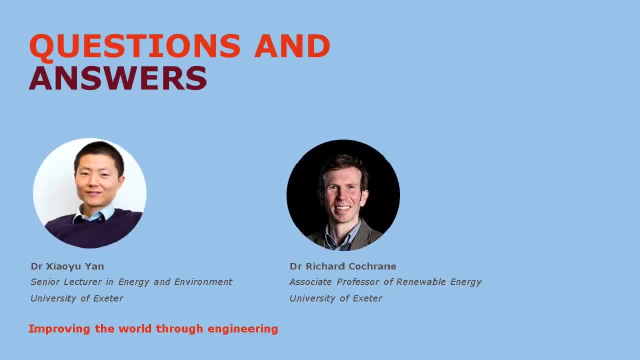 okay, i'm sorry. i guess there's still issues with some of the connections um, but i'll just try and pick up some of those questions. we're just looking at the list. steve roger's asked what's the typical lifespan of turbine blades. so they tend to be designed for um. 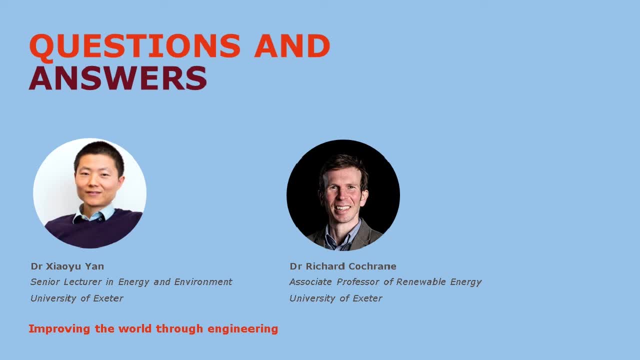 at least 20, 25 years. but that's based on certain wind characters, characteristics and, as I said, quite often there is opportunity to repurpose those blades and a lot of the turbines, where repowered, have been reused elsewhere. so, okay, Pandya has asked you know the recycling rate of wind turbine generators or other components. so 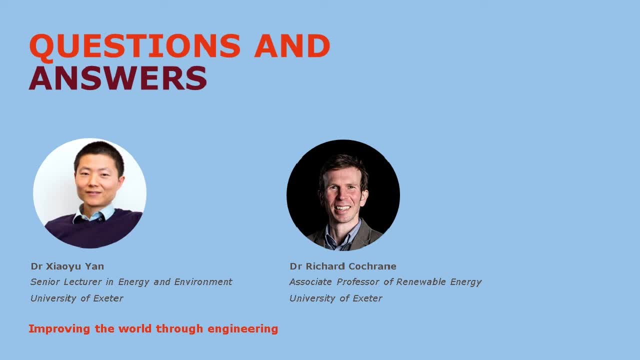 I think, yeah, generally those bits have been recycled very effectively. the metal components are far easier to process. separate out the copper from the steel and then they can be recycled very well. so good rate recycling rates on those components and the steel tower and other problems like that. Edward Cooper asked how wind turbine blades are used in a tidal energy system. 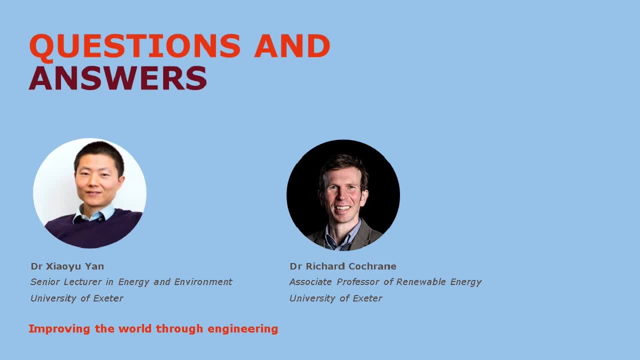 and well, there are different, quite different design drivers there, so if they often use similar components, then they can be recycled very effectively. so I think that's a good point. but the loading really is quite different and there are different design challenges, where it is particularly the weight of the blade that's an issue, but things like the pressure variation. 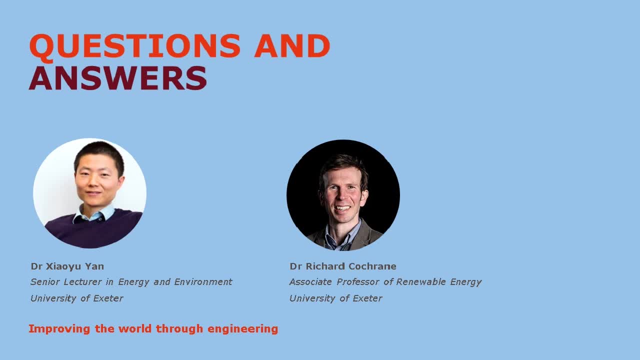 if the blade goes up and then goes down through the water cycle it's getting quite a lot of compression force, so often they're made far stronger, thicker, wall, that sort of thing to reduce that pressure difference, as opposed to a wind turbine blade which you're trying to minimize. 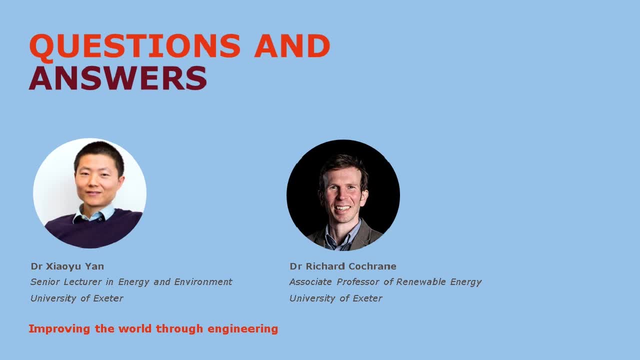 the weight very effectively, but certainly lessons learned and ways we can help and work together on that. Ruth has asked what's the cost difference between non-recyclable epoxy resin. that is the challenge I think at the moment is the volume of manufacture, the at the moment those recyclable. 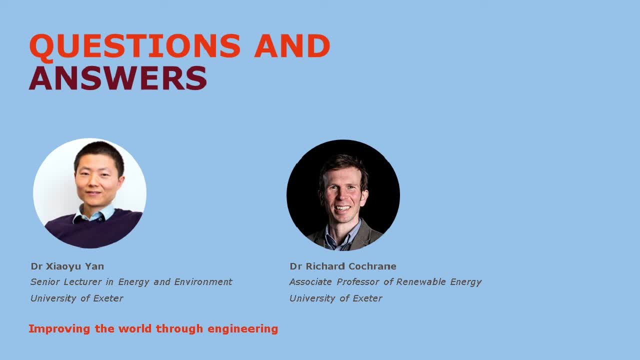 resins are novel as they come out of the wind turbine, but they're not as good as they used to be and only produced in relatively small quantities. so they are rather more expensive at the moment, but hopefully that will change in time going forward. industry certainly seems to be going. 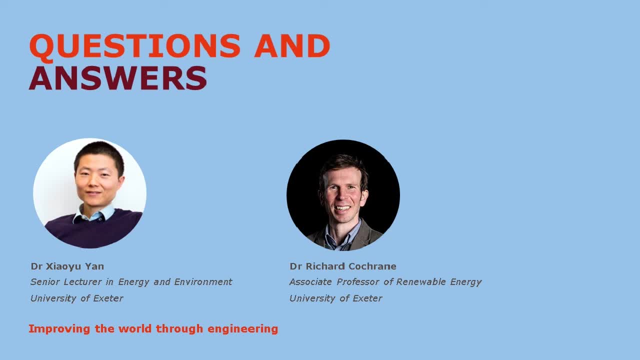 for that going forward. great, thank you and thank you. thank you, Richard, for taking over there. I do apologize. I seem to have dropped off the and dropped off the line there and it's just just come back in. so many many apologies for that and, Richard, thank you so much for. 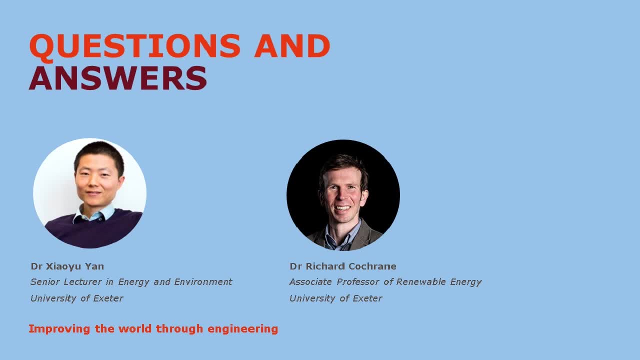 for jumping in and I just maybe wanted to pick up on on one question that have come in so I think particularly relevant, going going forward to COP 26. so one, one question here and I'll come to both, both of you, on this thing: do you have any thoughts on how governments should act now and how much is? 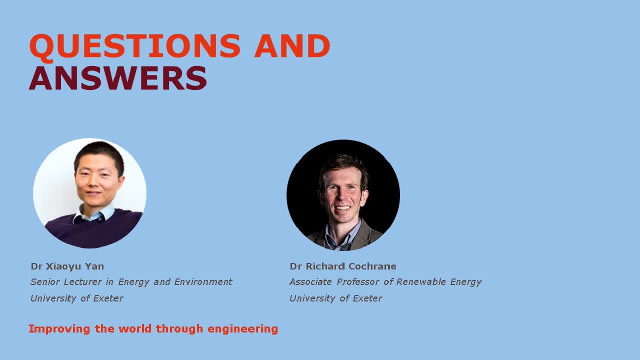 needed to offset our impact. perhaps, perhaps, which I could come come to you specifically thinking in terms of the wind industry, industry, what you might be looking for, and, again, I think that the support has been great, the push for particularly for offshore, but, um, there's still lots of. 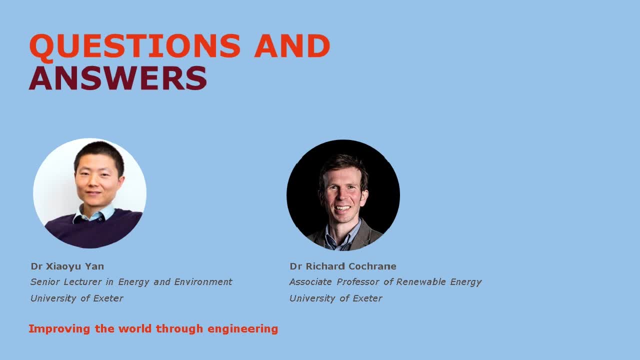 opportunities for onshore wind that are at the moment still more cost effective than than offshore, but that gap is closing quite impressively. um, a lot of that is related to planning rather than the energy technology going forward. but, yeah, support for R&D into developments like these. 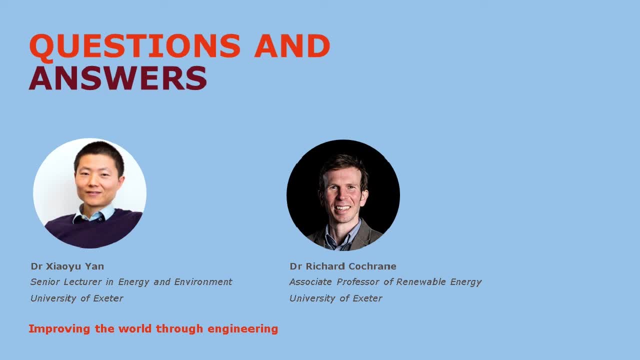 recyclable epoxies. those sort of things would be great to see supported. yeah, okay, that that's really. that's really helpful. thank you for your, for your thoughts, Matt and um, shall you perhaps just in terms of, uh, specifically in terms of life, life cycle analysis? 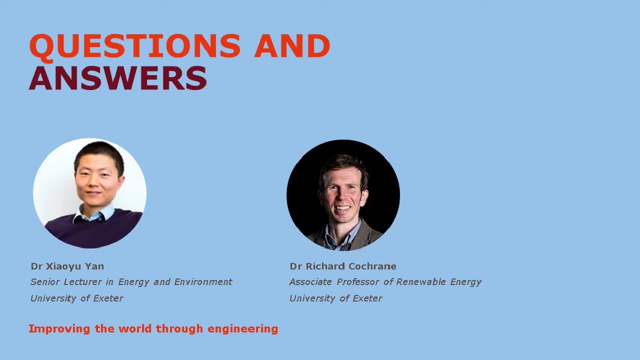 is there anything that you would be looking for you think that governments should do that could help us? um, yeah, it's a difficult question to answer because you can't do LCA on obviously everything. um, but I guess the the key kind of uh thing I want not just the government but but everyone, every one of us, to think about. 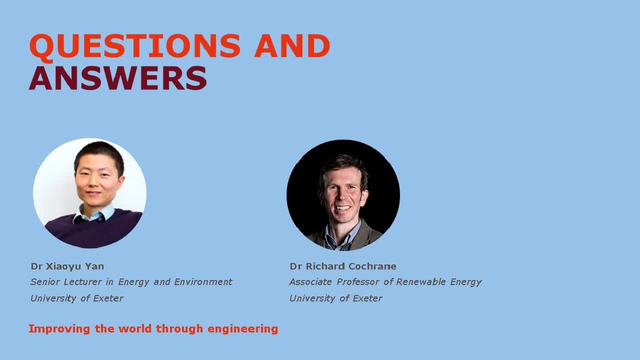 is that we don't just look at, uh, the apparent, uh kind of impacts. that's most visible essentially because we have to look at the whole life cycle and that means that that the most to me, that the most effective way of reducing life cycle impacts is actually reducing the consumption in the first. 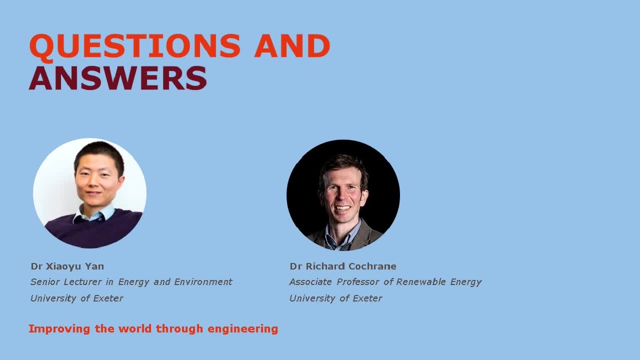 place um, because if we just keep um supply uh high using new technologies such as, you know, electric vehicles, Etc, yes, they're better than the conventional uh petrol and diesel cars, but over the life cycle they still have quite significant impacts. so what we should do is to try and reduce the demand for the cars. 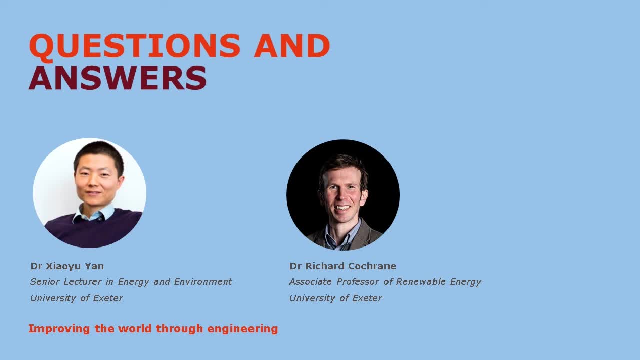 the driving, uh, in the first place, and the same goes for electricity as well. right, so the first thing is to to reduce the demand for electricity, and then we look at supply. uh, the rest with renewables, does that, does that answer? answer that question? yes, absolutely, yeah, no, that's really. 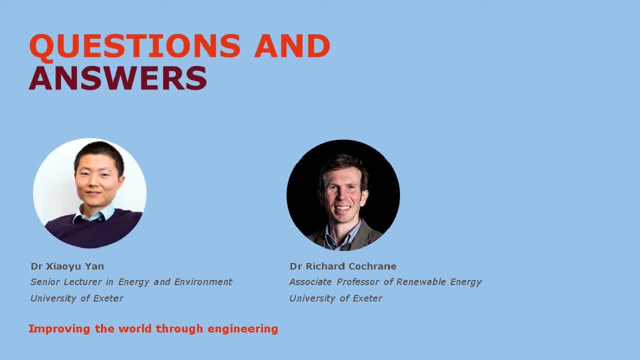 helpful, thank you. thank you very much, um, Richard. I just have another question for you, um, if that's okay. um, so there was just a question here in terms of- I think you may have partially answered this, but in terms of lifetime, uh, typically for the maybe blades and what would be the most determining? 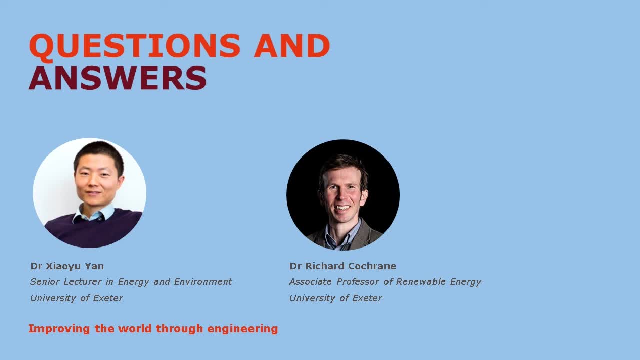 factors in for blade deterioration in terms of fatigue or corrosion or whatever the other major factors might be. yeah, so, yes, it is the time for 25 year life, but, as I said, some are being extended because they realize that they are more robust than they perhaps were designed to be um fatigue. 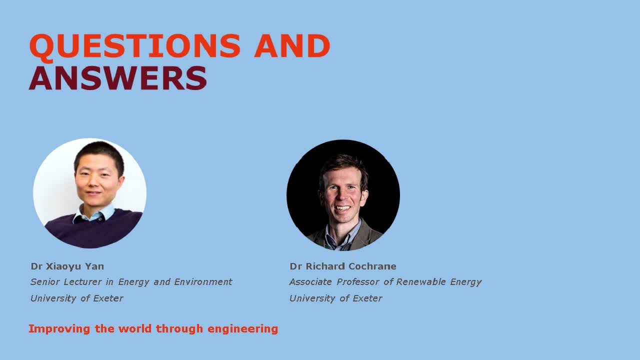 is the main driver in that the fatigue cycles blade, pulling one way or the other- I think that's one way- rotates around, pulls the other way. it pulls up, pulls around as well as the wind stopping and starting and those forces changing. so fatigue's main driver, other factors have influenced it. so 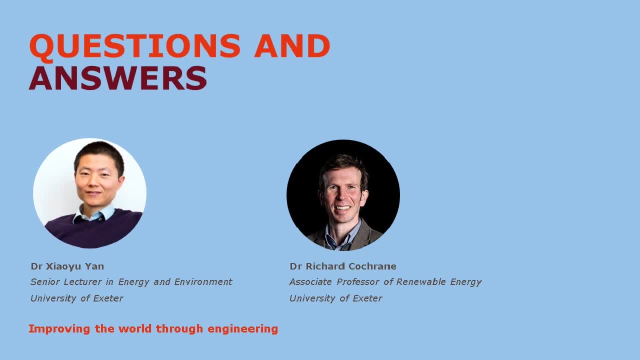 erosion, particularly in a sort of dusty environment, can take away the uh sort of gel coat, the outer layer of the um that's protecting the blade, and if water gets in that could damage things in a different way. but yeah, generally fatigue and those sort of life cycle is the 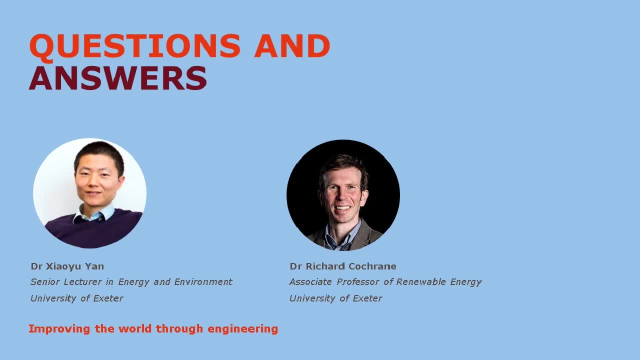 main driver for that, right. okay, thank you, um and I I. just one other question that's, I guess, come up, maybe just related to wind, in terms of the the life cycle cost of the wind turbine. um, is it sort of the build of your installation or the operation which is the sort of greatest driver? perhaps? I? 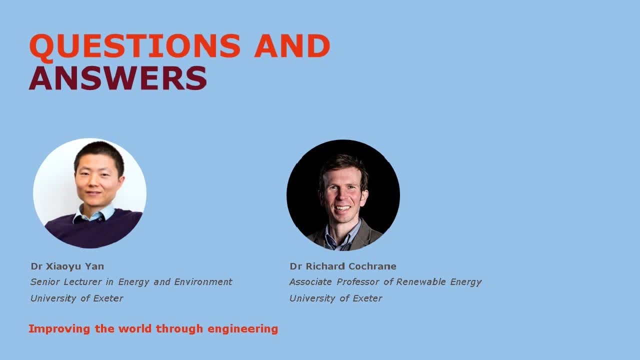 guess you're thinking most mostly of the co2 emissions. I don't know if either of you would be able to. to answer that question, I think yeah, in terms of co2. at the moment there is a lot of energy involved in the manufacturer and the assembly, but that is repaid. 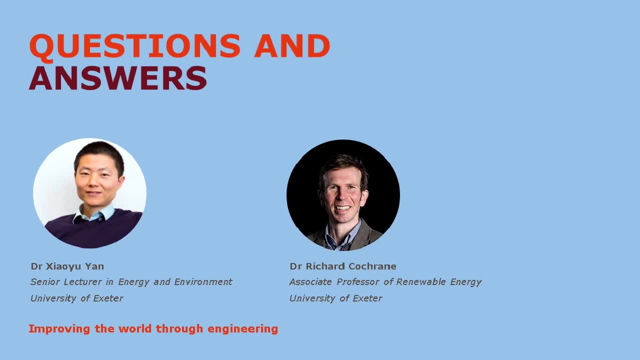 within six to nine months of the latest turbine developments. so quite impressive where they repay all that energy involved. on energy point of view, um cost wise, both both are important. so understanding the operational um aspects as well as the design work, both are important but a lot of. 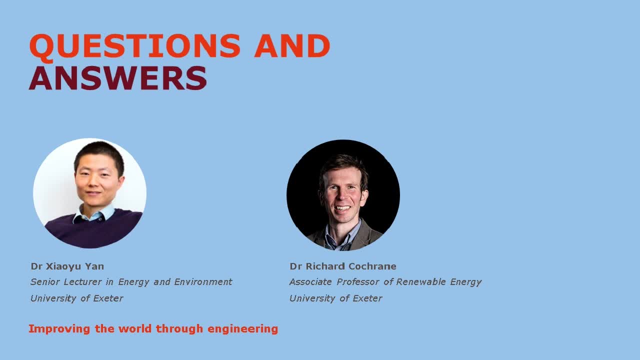 the cost is or the yeah, no, so both are very relevant. a lot of the improvements that we've made, particularly in offshore wind, has come from reducing the operational cost, making the turbines more reliable- so they have to be serviced, maintained less- and getting better at predicting when we need to go out and service that turbine- those sort of things. uh, has made the biggest. 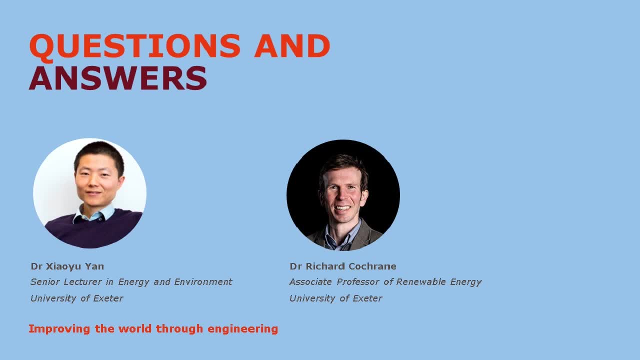 difference, I think, in the the cost, particularly for offshore wind. perfect, thank you. thank you so much, uh. thank you so much for that, Richard. we know that. I know that you have to um dash off to uh to a lecture now, so, um, I'll I'll give a few more questions to show you, but before you leave, Richard, 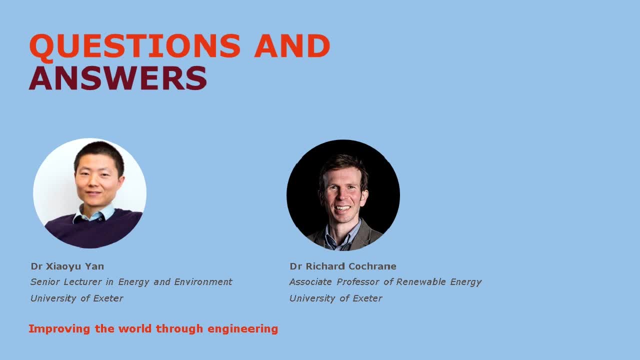 just from from my myself and from the Institute mechanical engineers, many thanks for for your, for your time and for this uh for the lecture today. thank you, Richard, no problem, thank you, it's been a pleasure and if there are other questions, my email address was on the slide, so very happy to. 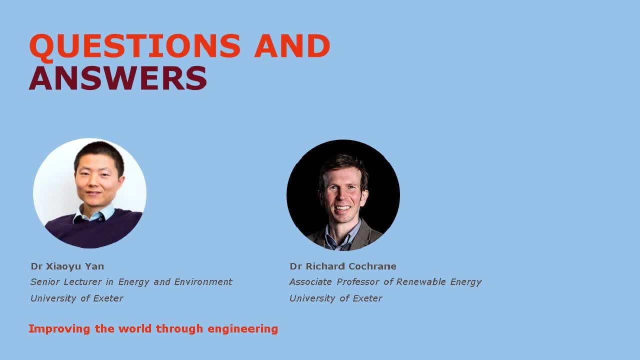 pick things up on the email if there are further questions that people want to ask. perfect, thank you so much. so you, I think you can stay with us for another couple of minutes. so, um, I did have a couple of LCA specific questions, which I just wanted to go through. one. one of the first ones that came in was: 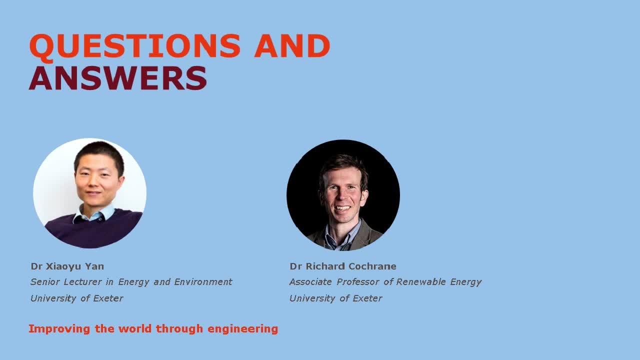 um. so our life cycle analysis: or is that mandatory? is that required um by government or or is that a sort of at the moment, is that an optional thing from manufacturers? um yeah, that's uh, actually mostly um optional or voluntary thing at the moment. different sections: um there are policies or regulations that require an LCA. 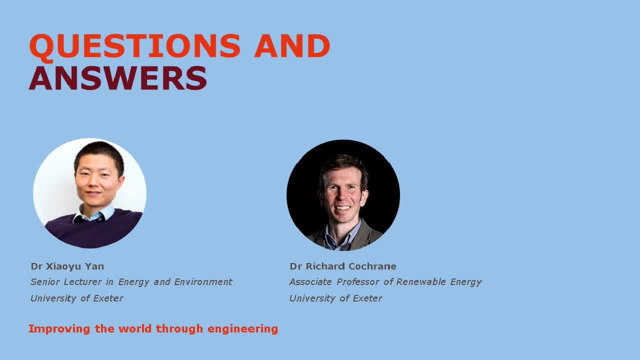 um is done so, for example, in the? um renewable fuels for transport uh sector. I believe that you have to show that the the type of fuel that you supply on the market have to meet a certain uh life cycle carbon footprint threshold, particularly for things like biofuels. voit. 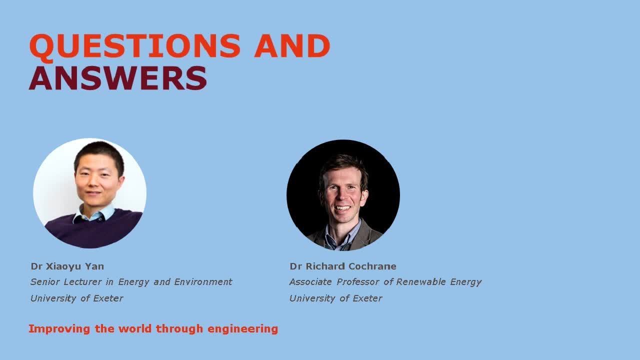 example, because some of the biofuels can be quite high carbon and it could be even more carbon intensive than the petrol and diesel that they replace. So you have to show that the biofuels that you supply on the market have to hit a certain 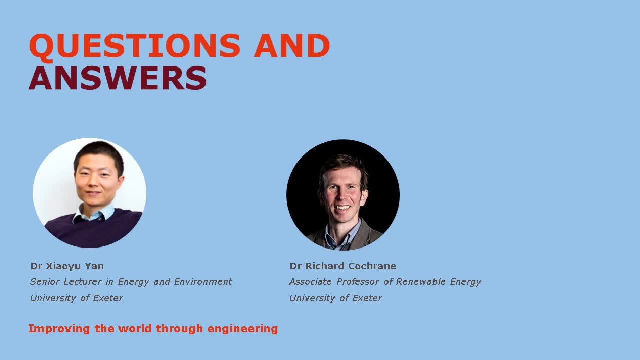 life cycle carbon footprint threshold. But apart from that, in terms of the energy industry, that's the only one that I'm aware of, So mostly it will be voluntary, really, Right, Okay, Understood that. I think that answers the question. 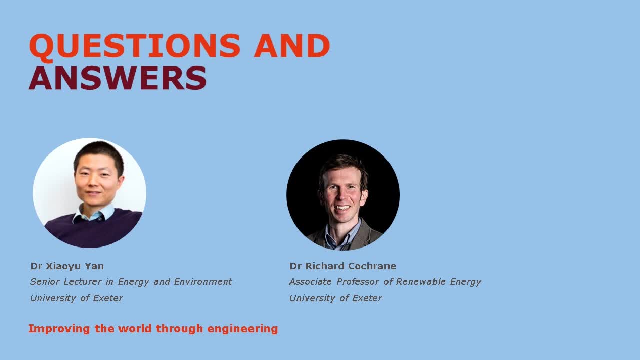 And then another one. I don't know if you could perhaps just briefly answer this, as we're a bit close on time, but so, in terms of comparing small-scale solar PVs- so domestic, maybe a solar panel on someone's roof- versus a sort of commercial installation, is there?